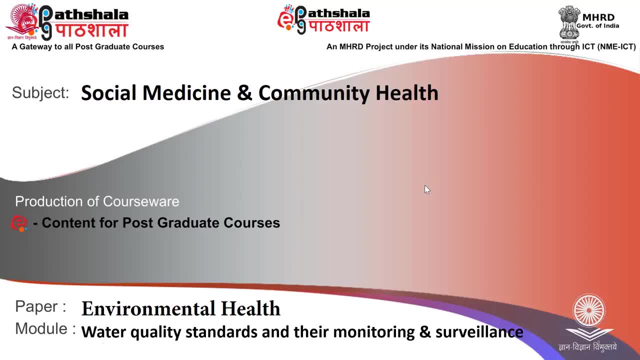 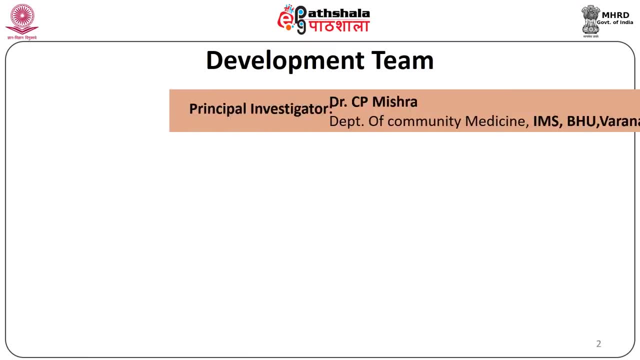 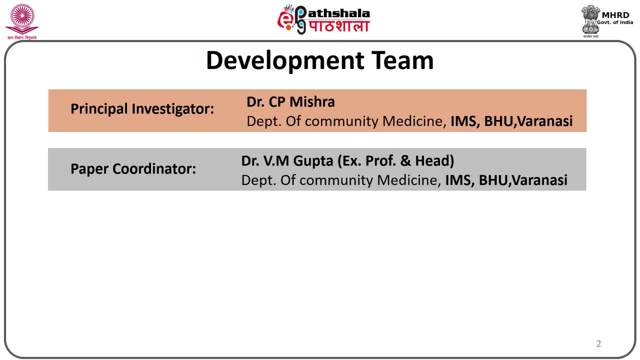 Monitoring and Surveillance. This module belongs to the paper Environmental Health. This has been developed by a team comprising of myself as Principal Investigator, Dr B M Gupta, Ex-Professor-in-Head Department of Community Medicine, Institute of Medical Sciences, Banasand. 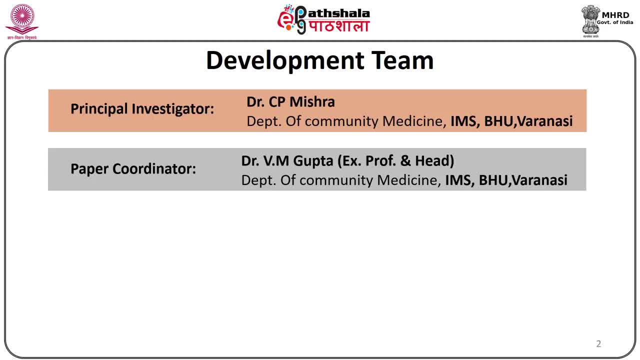 University, Varanasi, as Paper Coordinator. This module has been written by Dr Amit Kausik, from Department of Community Medicine Institute of Medical Sciences, Banasand University, Varanasi. as Paper Coordinator. This module has been reviewed by a team comprising of: 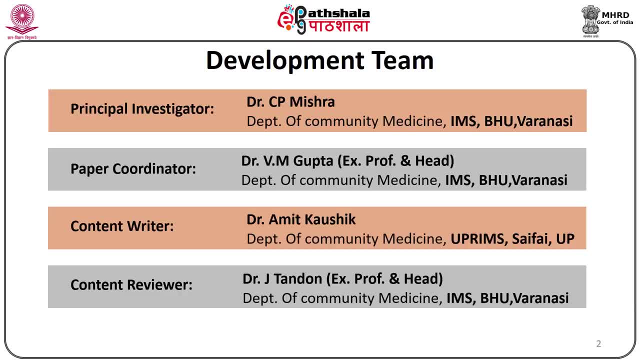 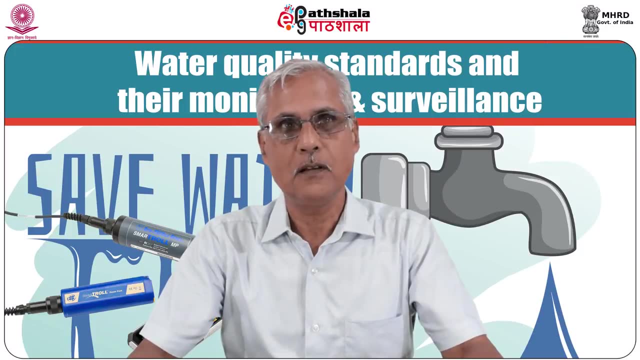 myself as Principal Investigator, Dr B M Gupta, Ex-Professor-in-Head Department of Community Medicine Institute of Medical Sciences Banasand University, Varanasi. The learning objectives that have been laid for this module is that one should be able: 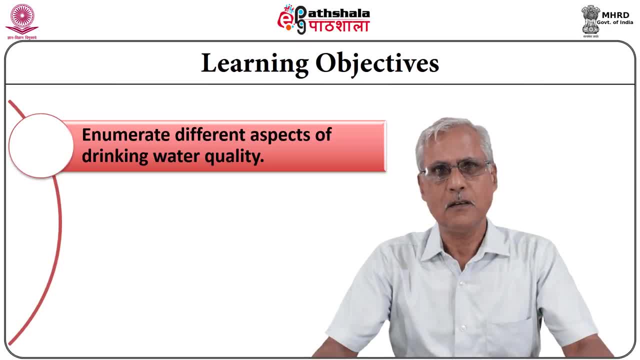 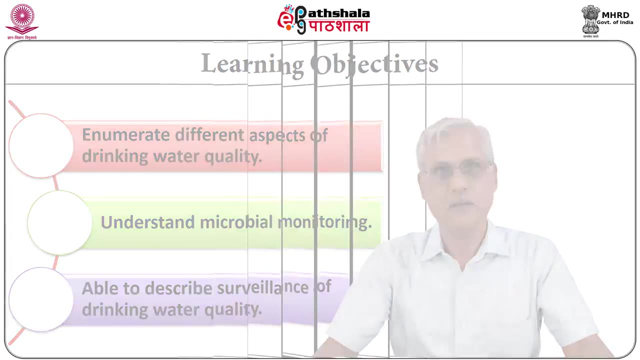 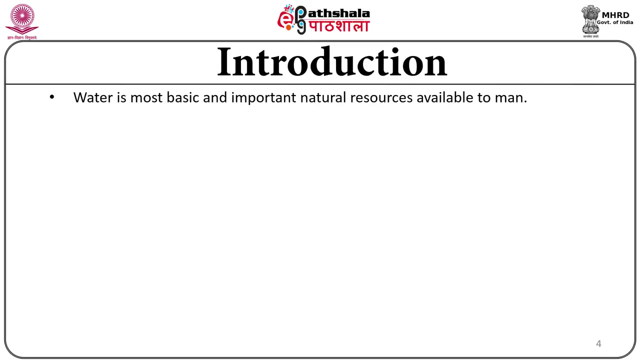 to enumerate different aspects of human health and can use this module to work out medical aspects of water quality, particularly with reference to drinking water. understand microbial monitoring able to describe surveillance of drinking water quality. we all know that water is the most basic and important natural resource available. 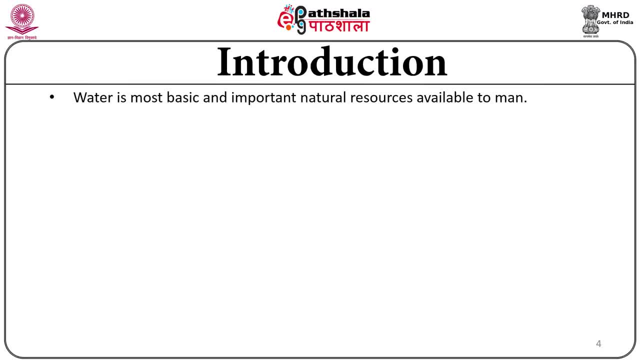 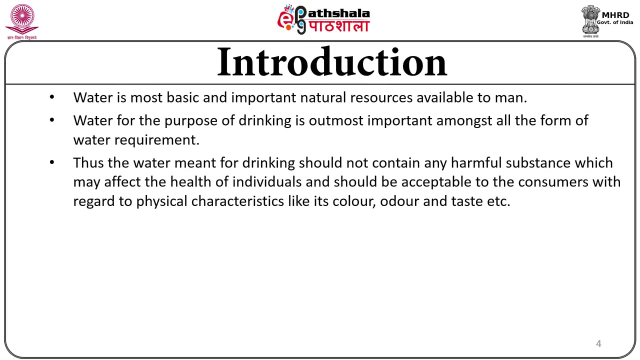 to man. they cannot be life it without water. water for the purpose of drinking is most utmost important among all. the form of water requirement does the water mean for drinking should not contain any harmful substance which may affect the health of individuals and should be acceptable to the 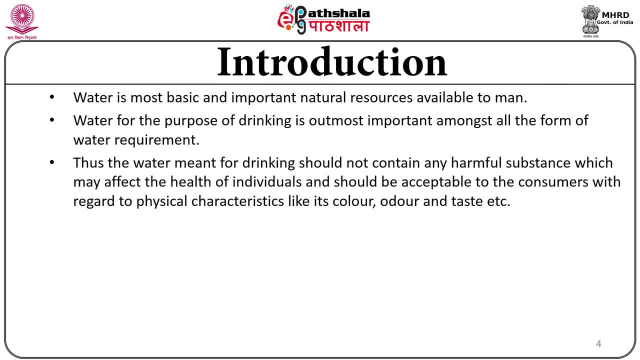 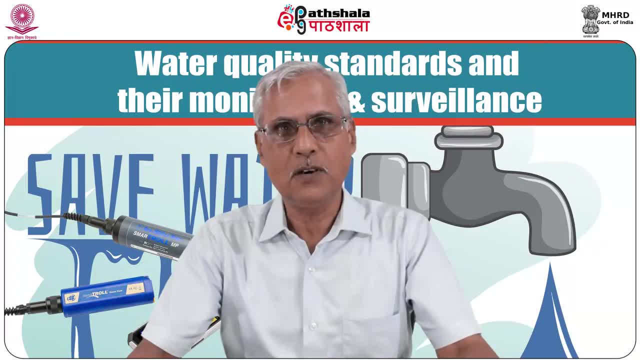 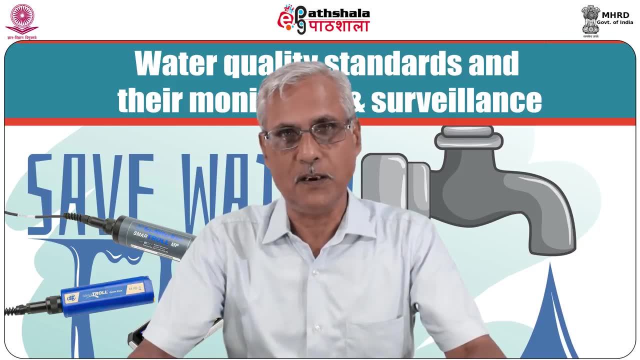 consumer with regard to physical characteristic, like its color, order and test. there should not be bacterial or chemical contamination of water and should be worth storing at household level. the risk of public health hazard is increased in case of failure of any single point of water supplies system, which includes sources of water. 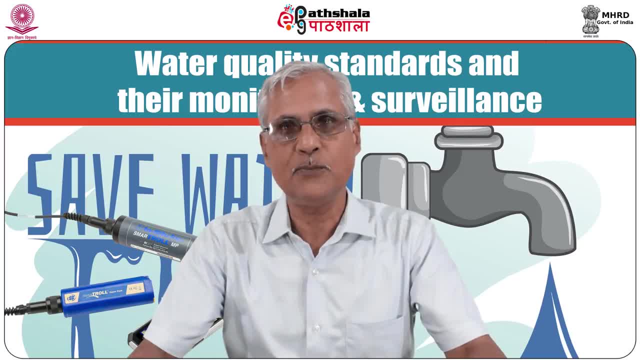 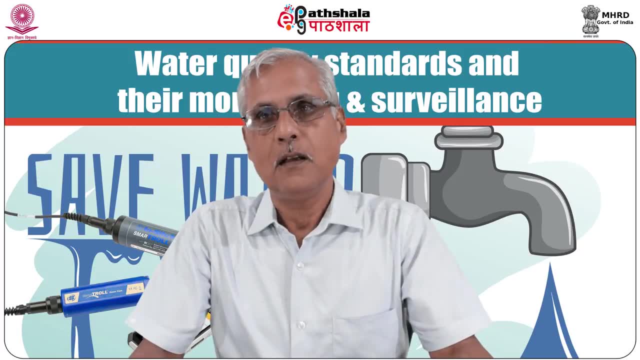 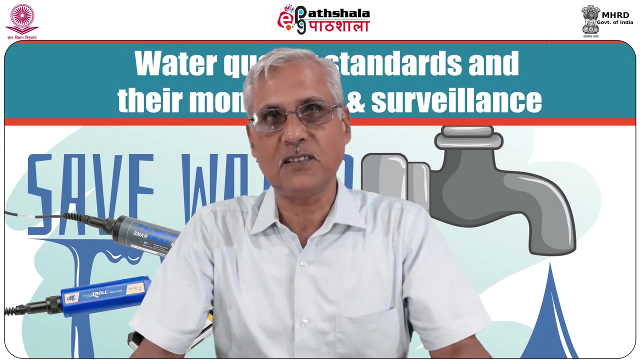 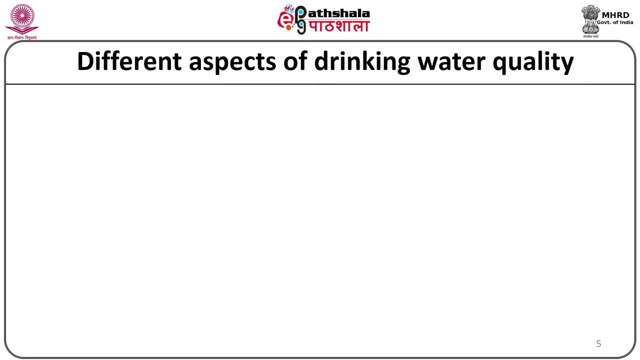 treatment processes, storage and distribution systems, although when there in the large-scale treatment process extra coordination is done, residual quality is kept at 0.5 ppm to take care of the problems. contamination that may occur through distribution systems and storage. different aspects of drinking water quality. as per WHO, that is one health organization- water quality: 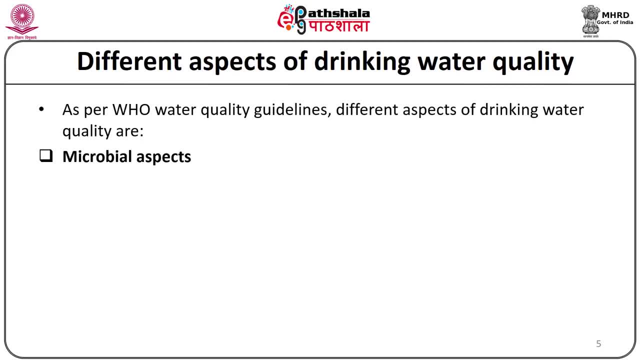 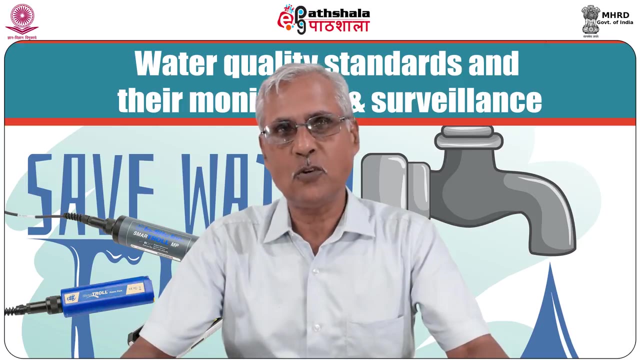 guidelines. different aspects of drinking water quality are: one is microbial aspects- that affects bacteria or organisms, virus, chemical aspects, radiological aspects, acceptability: accepts in terms of taste, order and appearance. as for as microbial aspect of drinking water quality is concerned, the greatest risk to health is imposed by fecal matter of human as well as animals. 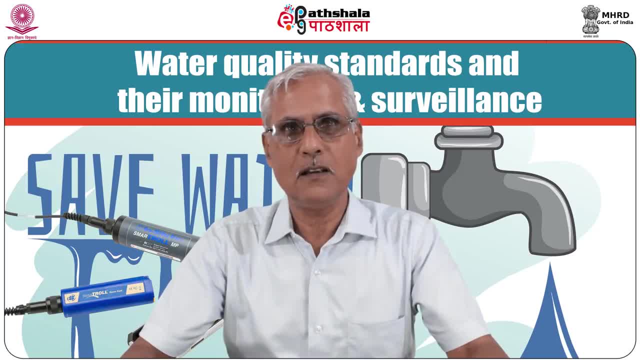 fecal matter can be a source of number of pathogenic microorganisms, including bacteria, viruses, protozoa and helminthes. not only the pathogens from fecal matter, but other microbial hazards like guinea worm, which have been now eradicated from source waters, and ligonilla. 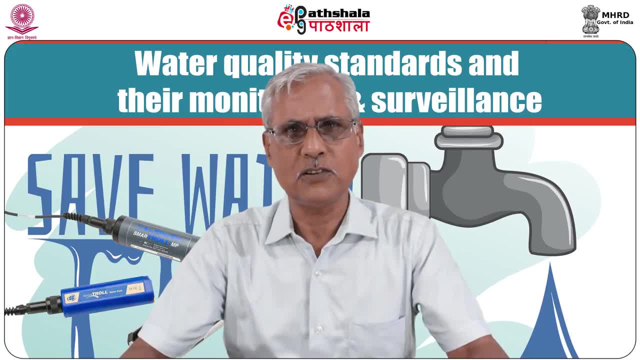 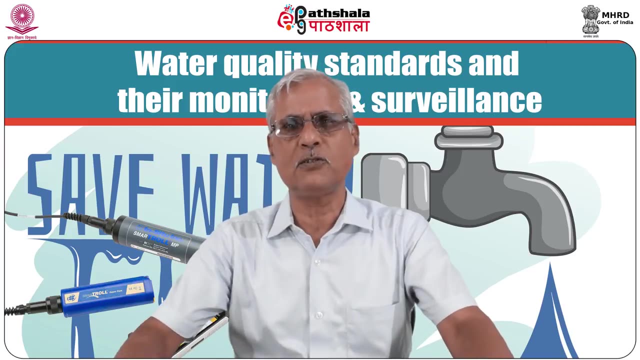 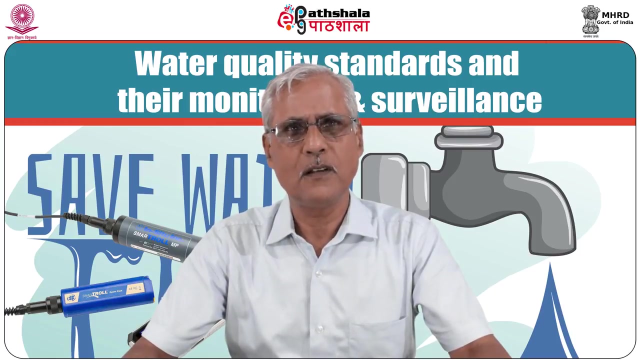 now in pipe water distribution system, also associated with it. Attributable factors for the public health burden associated with consumption of contaminated water, severity and incidence of illnesses associated with pathogens, their infectivity and the population exposed. various routes involved are ingestion, one of the important. 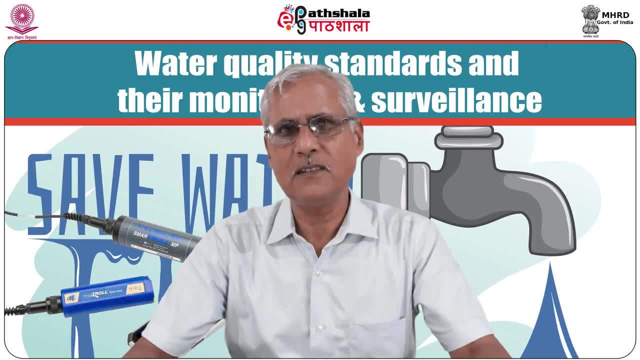 thing is like Campylobacter species, Scacea coli, Salmonella species, Cegla species, Bebrioculera, Hepatitis A virus, Hepatitis B virus, Intermebiva Asterolytical and GRD in test analysis. 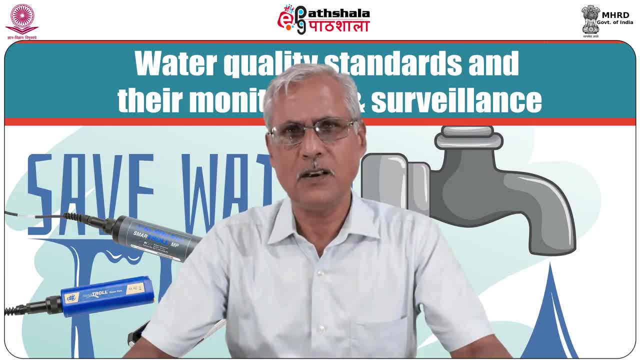 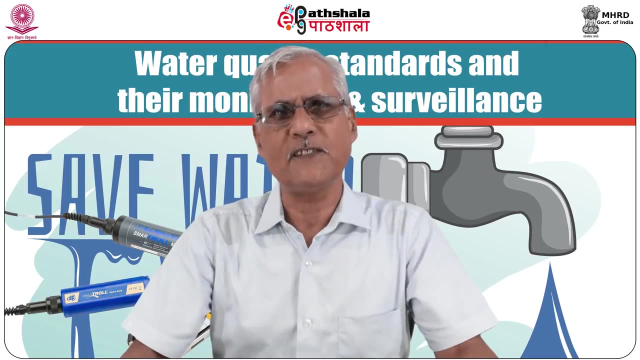 Inhalation adenoviruses, Enteroviruses, ligonilla pneumophila or by direct contact during bathing. Acanthomebiva species, Burkholderia Pseudomeli, Leptospira species. Reference pathogens: adenoviruses, Adrenoviruses- Adrenovirus Adrenovirus- Adrenovirus Adrenovirus. 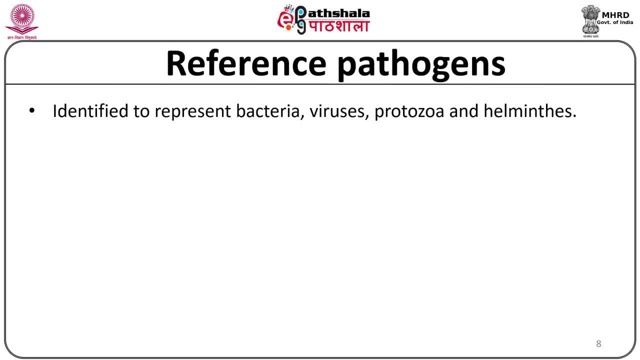 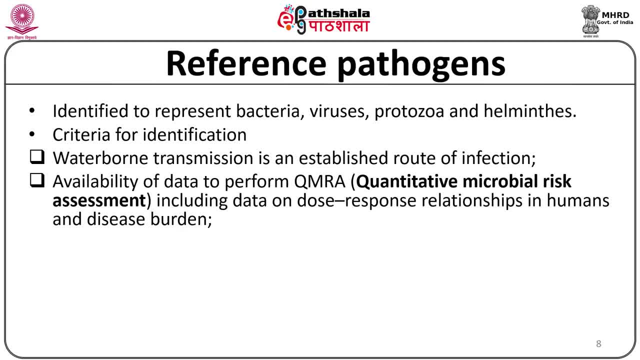 Availability of data to perform quantitative microbial risk assessment, including data on dose response resistance in humans and disease burden, Occurrence in source waters, Persistence in the environment And sensitivity to removal or inactivation by treatment process, Infectivity incidence and severity of disease. 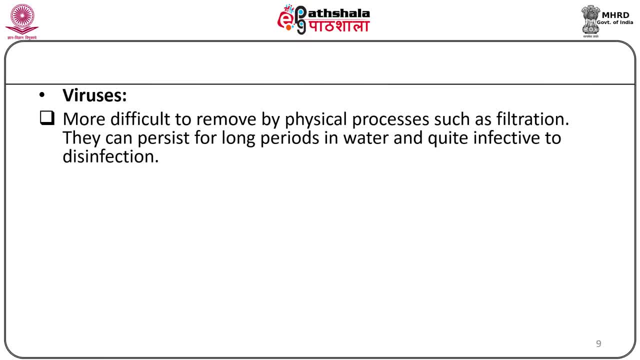 Viruses more difficult to remove by physical process such as filtration. They can persist for long periods in water and quite infective to disinfection. Rotaviruses, enteroviruses, noroviruses have been identified, Potential reference pathogens. 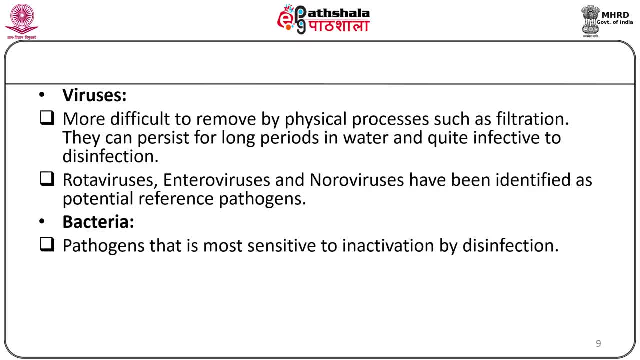 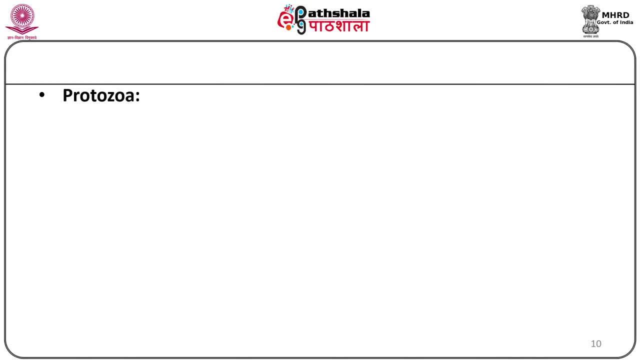 Bacteria Pathogens that is most sensitive to inactivation by disinfection Dose response models are available for Vibrio Compylobacterium E, Coli 0157,, Salmonella and Sigla Protozoa. 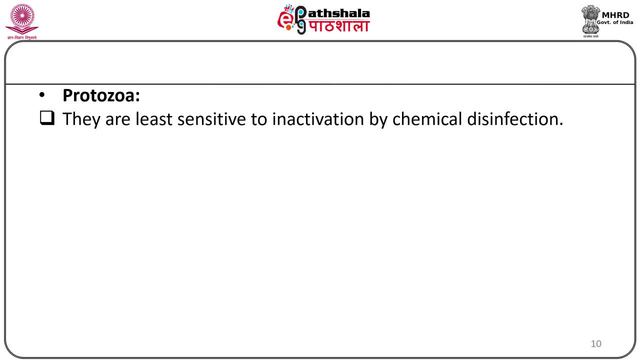 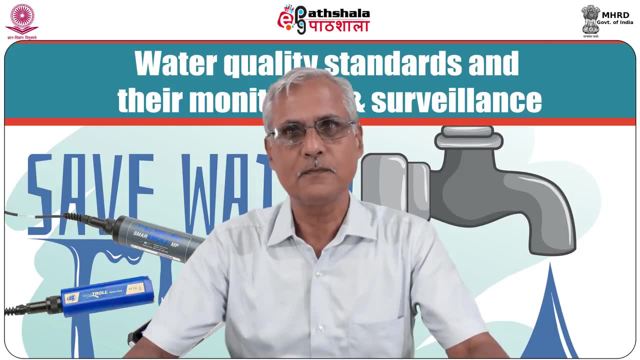 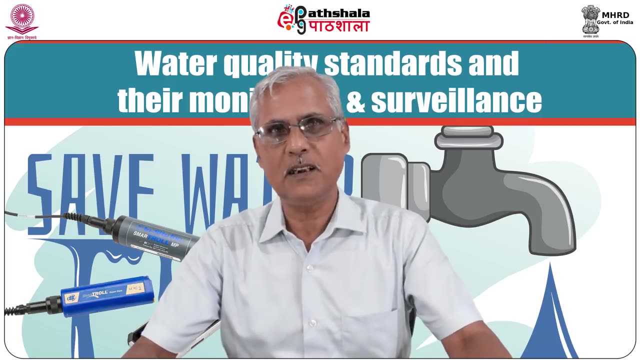 They are least sensitive to inactivation by chemical disinfection. Dose response models are available for Giardia and Ketoplasma Heptospiridum. VM- Quantitative microbial risk assessment- QMRA Systematically combines available information on exposure. 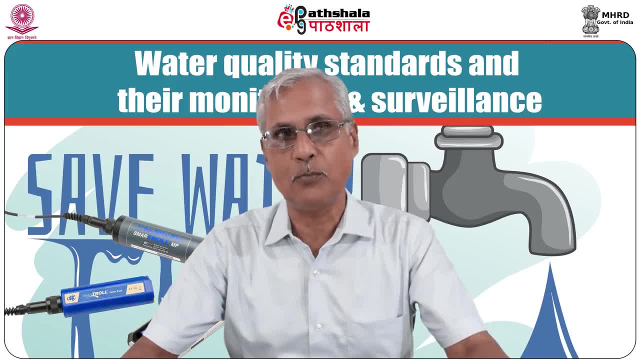 The number of pathogens ingested And dose response models to produce estimates of the probability of infection associated with exposure to pathogen in drinking water. Microbial monitoring Indicator organism is needed for monitoring Criteria for fecal indicator Inversely present in feces of human and animals. 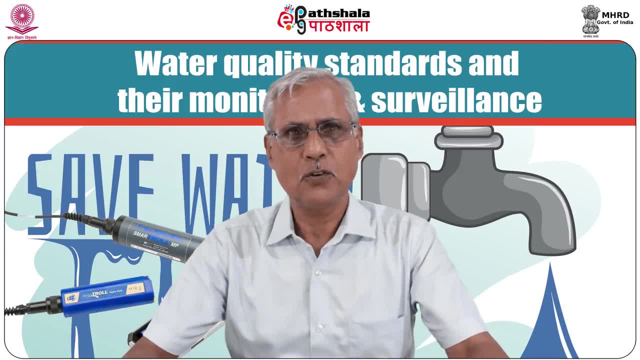 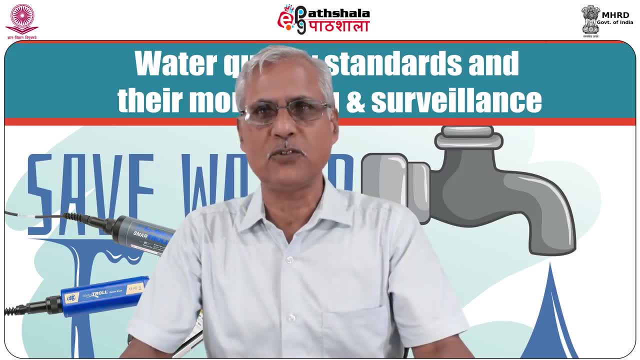 Should not multiply in natural water. Should persist in water in a manner similar to fecal pathogens And should be present in higher numbers than fecal pathogens. Should respond to treatment process in a similar fashion to fecal pathogens. Should readily be detected by simple inexpertise. 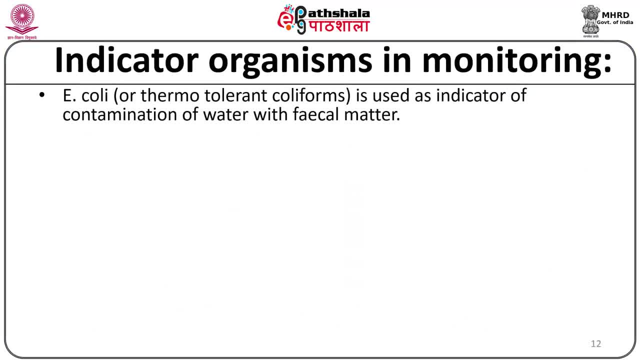 Cultural methods. Integrated organism monitoring. E coli or thermotolerant coliforms is used as an indicator of contamination of water with fecal matter. Total coliforms indicate the cleanness and integrity of distribution system. Helicotrophic plate count indicates effectiveness of disinfection process and cleanness. and. 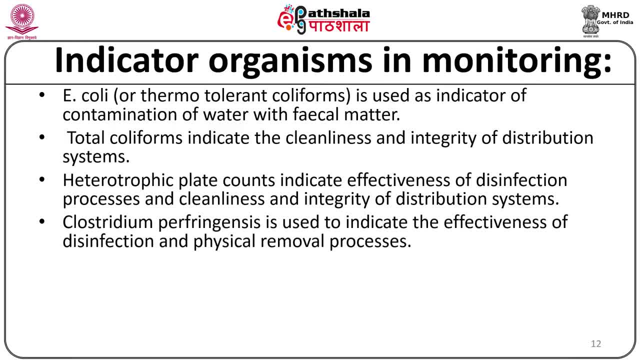 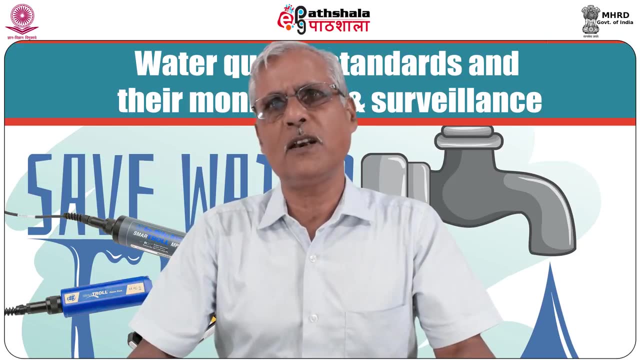 integrity of distribution system. Clostridium perfringensis is used to indicate the effectiveness of disinfection and physical removal processes. Enteric viruses as indicator of effectiveness of disinfection and physical removal process for viruses. Guideline values for verification of microbial quality. 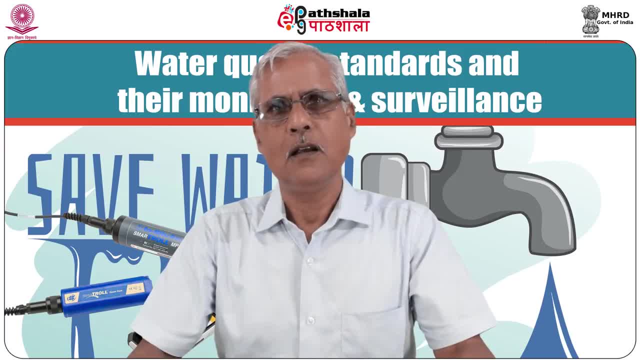 This is again by World Health Organization Organism guideline value: All water directly intended for drinking. E coli or thermotolerant coliform bacteria must not be detected in any 100 ml of sample Treated water entering the distribution system E coli or thermotolerant coliform bacteria. 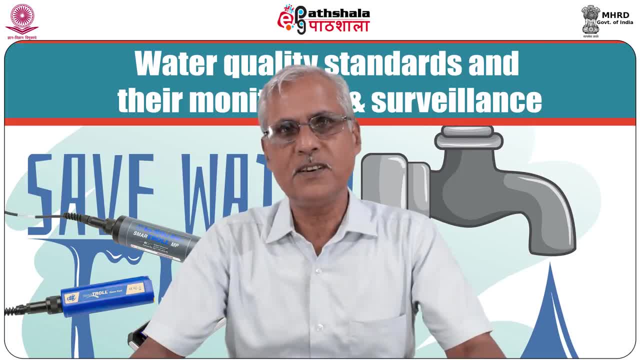 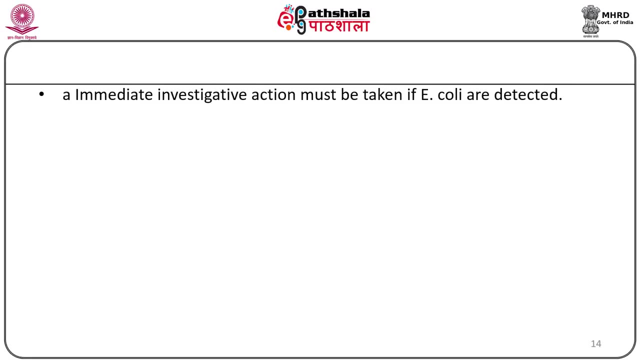 must not be detected in any 100 ml sample Treated water in the distribution system. E coli or thermotolerant coliform bacteria must not be detectable in 100 ml of sample. A immediate investigation action must be taken if E coli are detected. 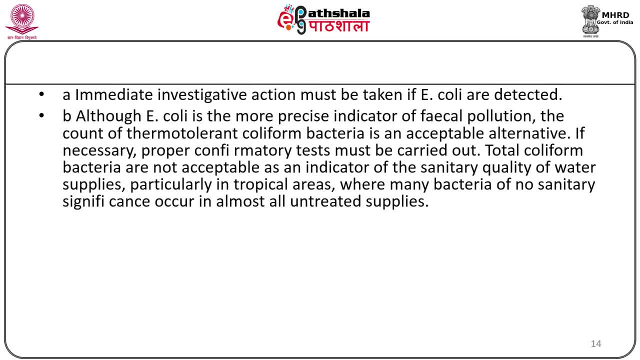 B. Although E coli is the more precise indicator of fecal pollution, the count of thermotolerant coliform bacteria is an unacceptable alternative. If necessary, proper confirmatory test must be carried out. Total coliform bacteria are not acceptable as indicator of solitary quality of water. 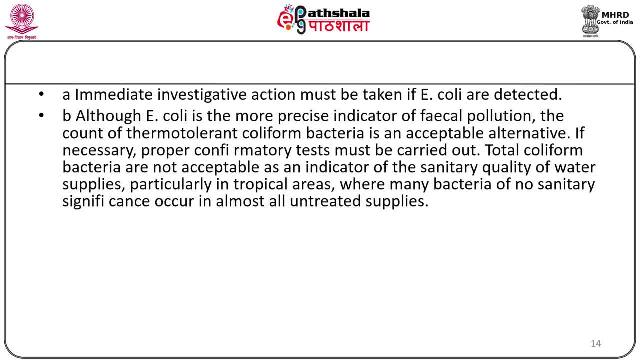 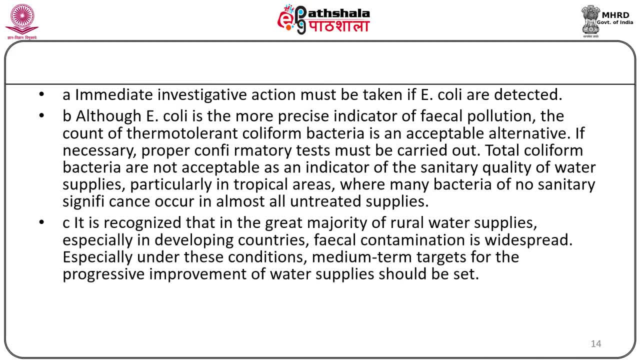 supplies, particularly in tropical area, where many bacteria of no solitary significance can occur in almost all water. This is the end of this video. Thank you for watching, See, it is recognized that in the great majority of rural west supplies, especially in developing countries, fecal contamination is widespread, especially under these conditions: medium 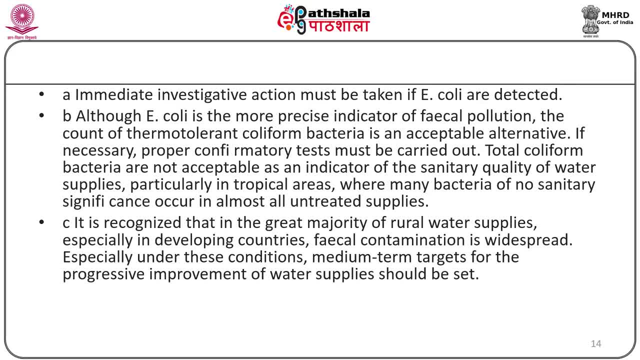 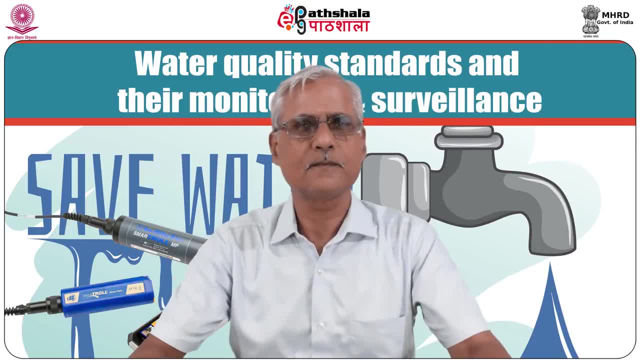 term targets for progressive involvement of water supply should be set. The second aspect is chemical aspects. The chemical constituents have Ability to cause adverse health effects after prolonged periods of exposure which summed by a single exposure through massive accidental contamination of drinking water supply. Categorization of source of chemical constituents: source of is again world health organization. 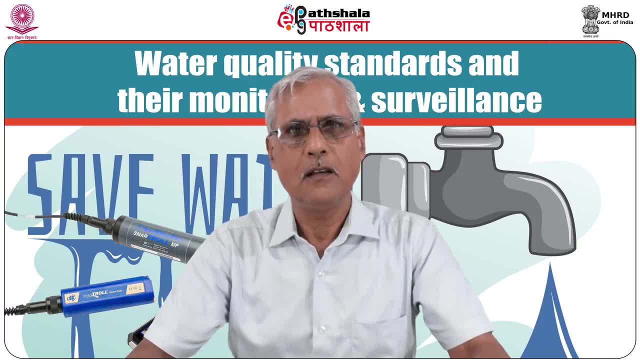 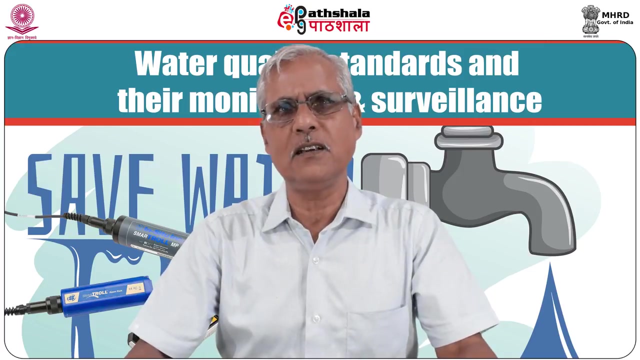 mainly five types: naturally occurring chemical constituents. Industrial sources and chemical constituents And human dwellings. agricultural activities related chemicals, water treatment or materials in contact with drinking water. naturally occurring, found mostly in rocks, soils and the effects of geological setting and climate. eutrophic water bodies, also influenced by serious inputs. 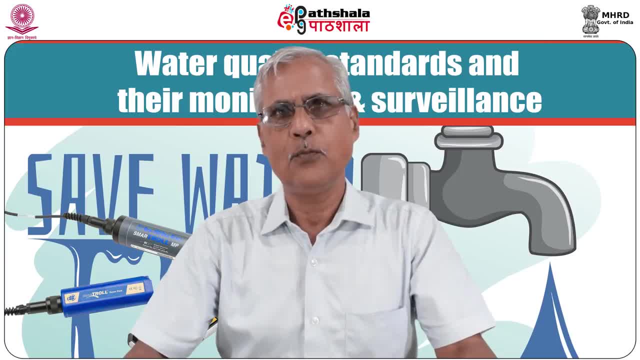 and agricultural runoffs. Examples are arsenic, barium, boron, chromium, fluoride. So these are some of the most common examples of geological activities related to geological setting and climate. eutrophic water bodies are also influenced by serious inputs and agricultural runoffs. 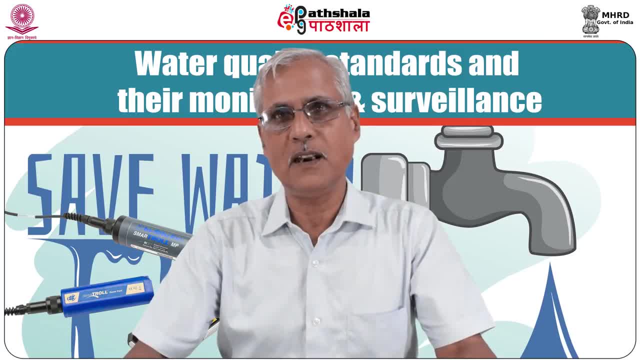 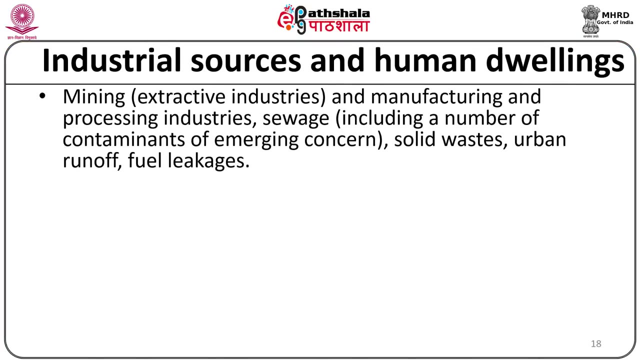 Examples are arsenic, barium, boron, chromium fluoride, Selenium, colloid hardness, hydrogen, sulfide, iron, manganese, molybdenum. pH of water, sodium, potassium, sulfate. total dissolved solids. Industrial sources and human dwellings, mining, extractive industries and manufacturing and processing industries. sewage, including a number of contaminants of emerging concern. solid. 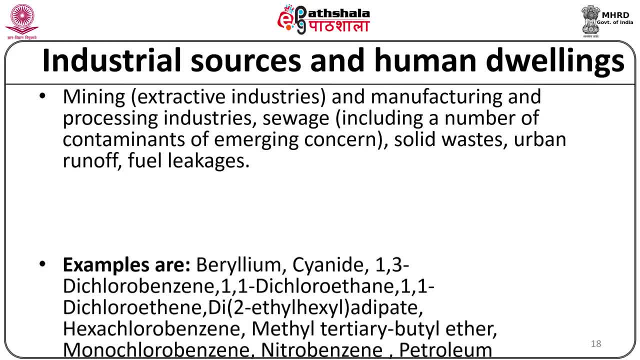 beds, urban runoffs, fuel leakages and so on. Examples are beryllium, cyanide, 1,3-dichlorobenzene, 1,3-dichloroethane, 1,1-dichloroethane, di-2-ethyl-hexyl-adipate. hexachlorobenzene, methyl tersky-butyl ether, monochlorobenzene, nitrobenzene, petroleum products and trichlorobenzene 1,1-1-trichloroethane. In number of industrial sources, we can say that the most common sources of geological activity related to climate. eutrophic water bodies are manganese, boron, chromium, fluoride, chlorobenzene and so on. Examples are beryllium, cyanide, 1,3-dichlorobenzene, 1,3-dichloroethane, 1,1-dichloroethane. 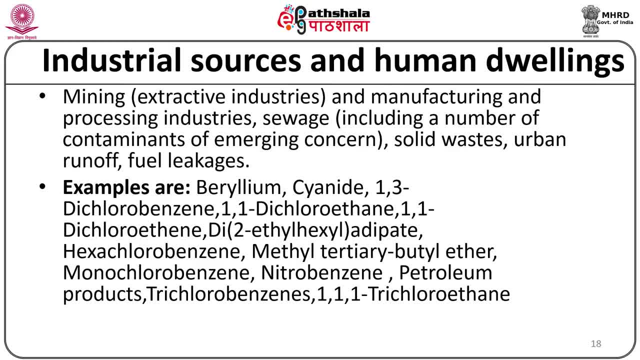 di-2-ethyle-hexyl-adipate, hexachlorobenzene, methyl tersky-butyl ether, monochlorobenzene, nitrobenzene, petroleum products and trichlorobenzene 1,1-1-trichloroethane. 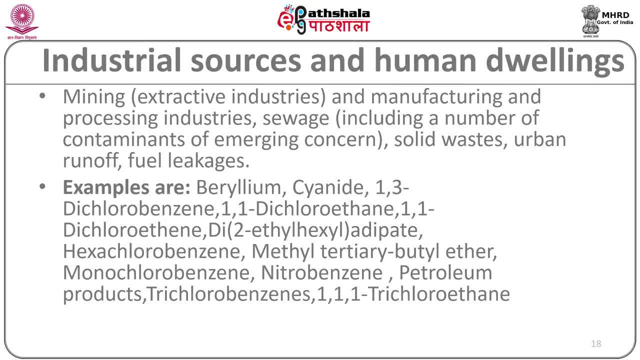 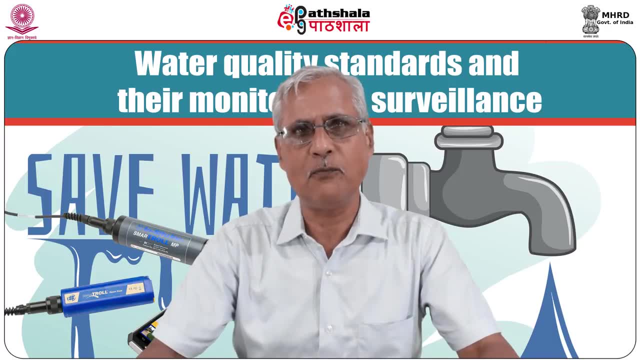 5. A number of agricultural activities, from manures from fertilizers, internship animal practices to data and such studies linked to different adelphian fecal君, TL, TCO and EGLI, моей, idempitens and other biology field aspects are found in the list of bases. 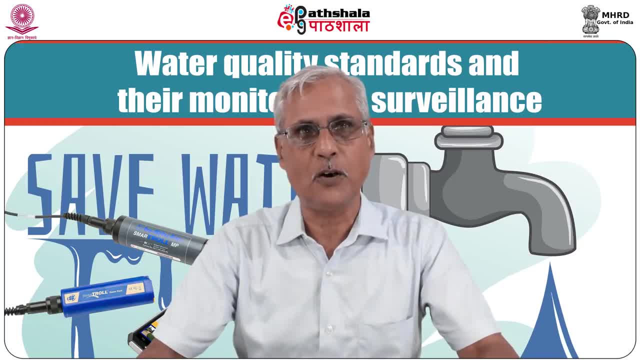 표 ráp. Seoulrament infiltrates an俺onzon and pesticides. they pollute water bodies. there are three types: inorganic cadmium and mercury. organic benzene, carbon tetrahydride, 1, 2 dichlorobenzene and nitric acid. non pesticides. 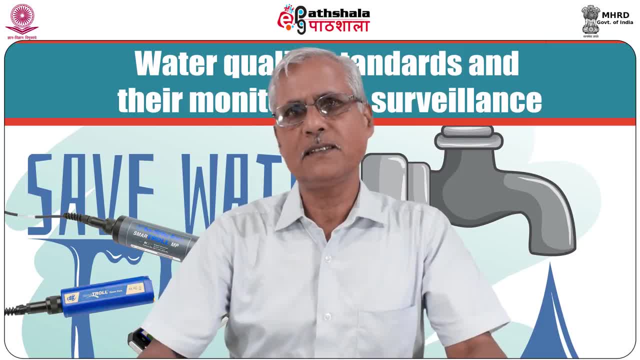 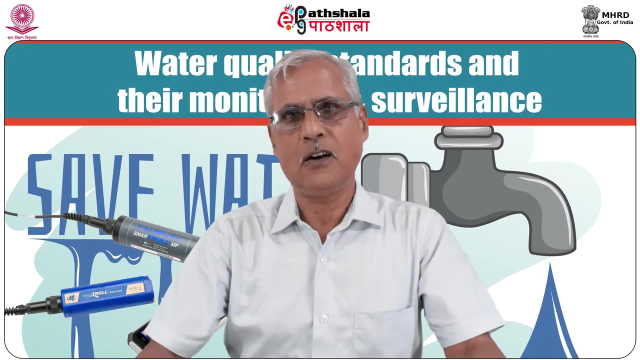 nitrates and nitrites. nitrates, nitrates, high level of nitrates indicate recent pollution, and high level of nitrate indicates old pollution or old contamination with physical matter. pesticides used in agriculture: aldicar, aldrin, dialdrin, linden, methoxychlor and so on. 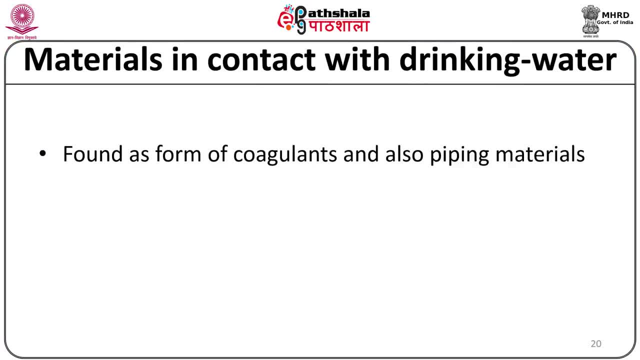 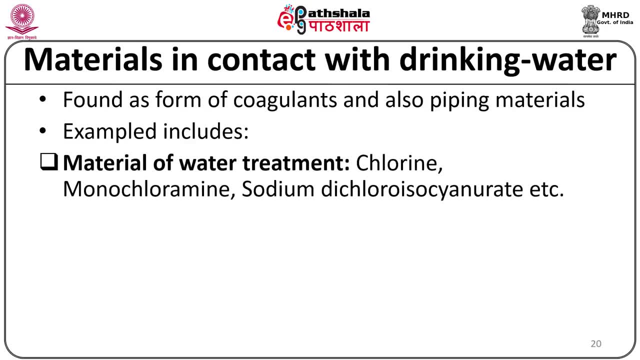 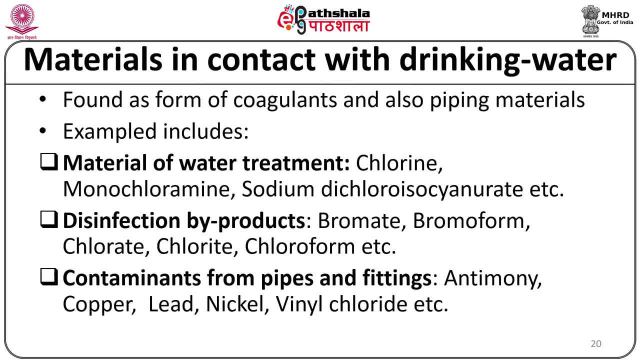 materials in contact with drinking water, found as form of coagulants and also piping materials. examples include material of water treatment, chlorine, monochloramine, sodium dichloro, iso cyanurate. disinfection by products, bromate, bromoform chlorate, chlorite, chloroform. contaminants from pipes and fittings like antimony, copper, lead, nickel, vinyl chloride. 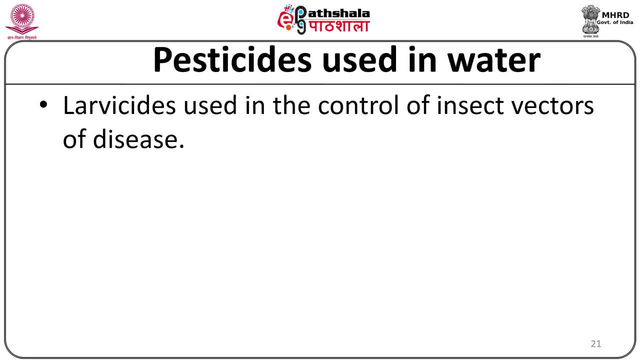 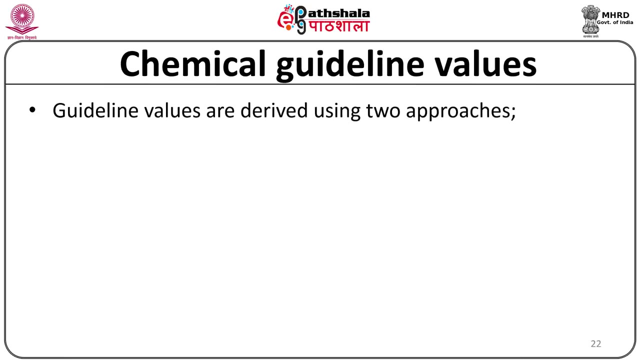 pesticides used in water. larvicides used in the control of insect vectors of disease. examples are diflubene, benzoyl monon, methoprin, lobeleran, imifos, methyl pyroxifen and temifas. the guidelines for chemical guidelines values are guidelines. values are derived using two approaches: threshold. 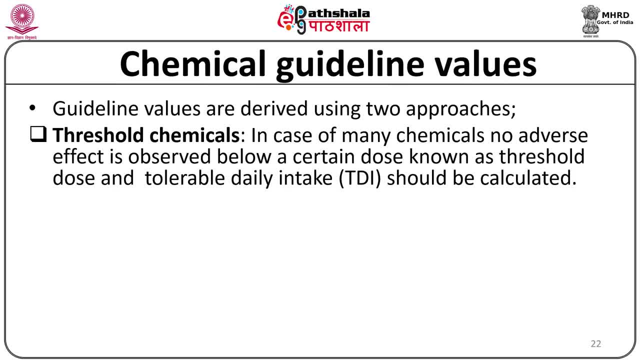 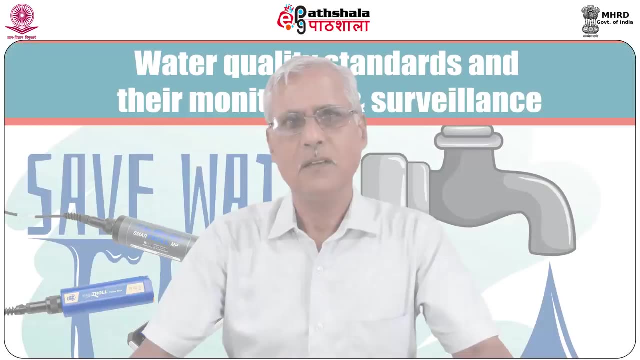 chemicals. in case of many chemicals, no adverse effect is observed below a certain dose, known as threshold dose and tolerable daily intake- tdi- non-threshold chemicals. these are mainly genotoxic carcinogens. models are used to develop guidelines values for those. these models compute an estimated of risk at a particular level. 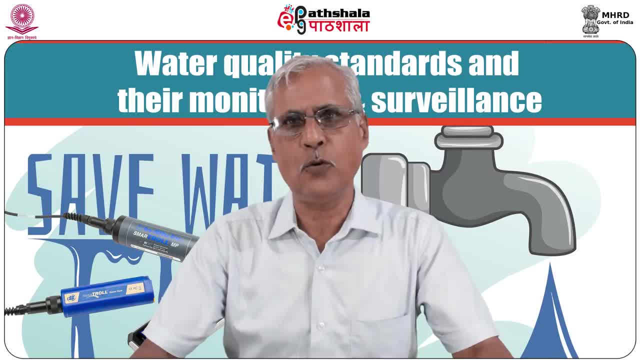 of exposure, along with upper and lower confidence limits. tolerable daily intake is identified by method of gradient analysis of a variable level of exposure to the load of the top to. It is an estimate of the amount of a substance in food and drinking water exposed on a body. 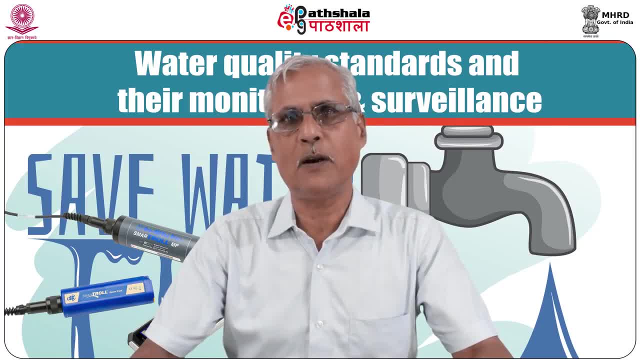 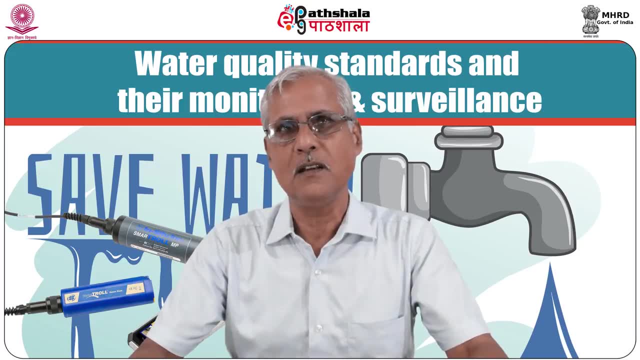 weight basis milligram or microgram per kilogram of body weight that can be ingested over a lifetime without appreciable health risk and with a margin of safety So tallable. daily intake is calculated taking into account the lifetime risk without appreciable 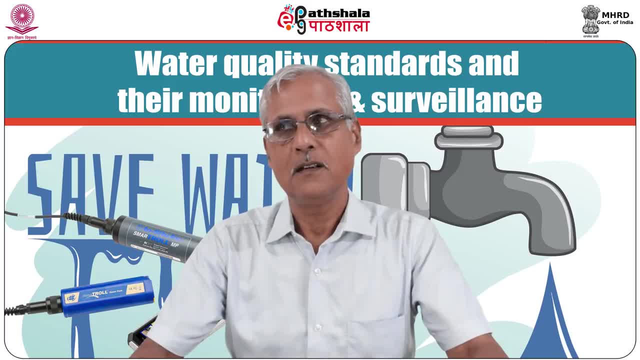 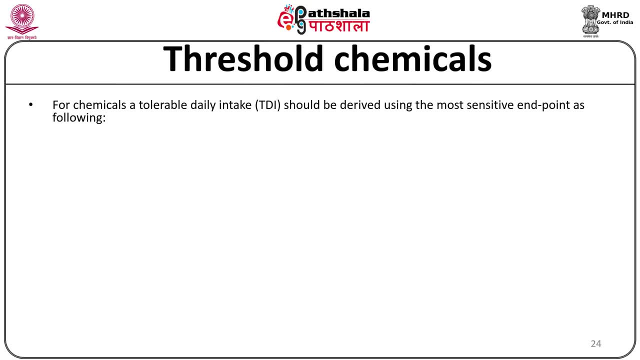 health risk and with a margin of safety Threshold, chemicals are. for chemicals, a tallable daily intake should be derived using the most sensitive endpoint as following: TDI is equal to NOAEL or LOAEL or BMDL, UFL or CSAF, where. 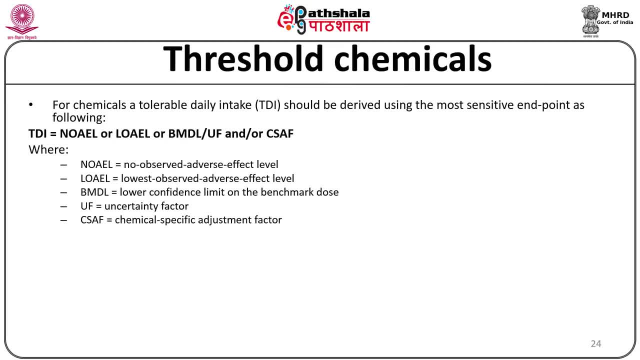 NOAEL is low observed adverse effect level. LOAEL is lowest observed adverse effect level. NOAEL is low observed adverse effect level. LOAEL is lowest observed adverse effect level. BMDL, lower confidence limit on the benchmark dose and UF means uncentred defactor and CSFA. 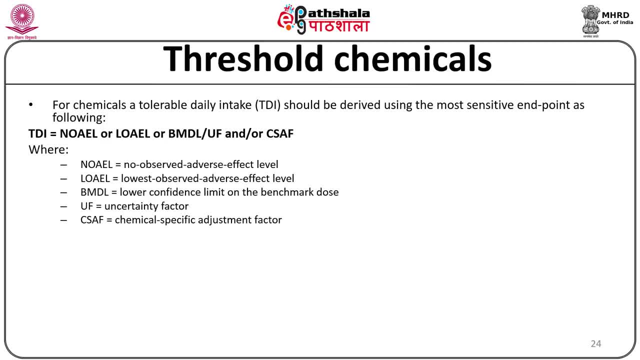 chemical specific adjustment factor. So TDI takes into cognizance these ah values. The guideline value is then derived from TDI as follows: GV equal to TDI into BW, into P, by C, Where BW is body weight, P is fraction of the TDI allocated to drinking water and C is 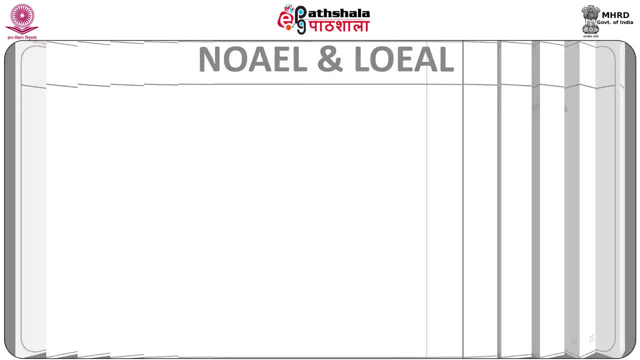 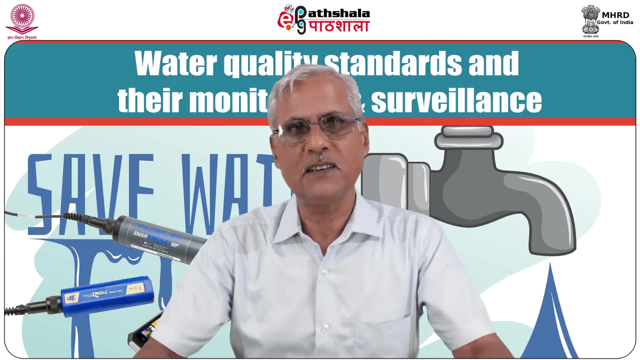 daily drinking water consumption. NOAEL and LOAEL. the NOAEL is defined as the highest dose or concentration of chemical that cause causes no detectable adverse effect and if NOAEL is not available, LOAEL lowest observed dose or concentration of substance as which a detectable adverse effect occurs. 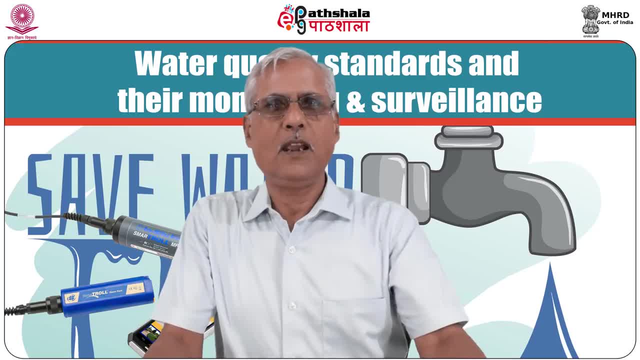 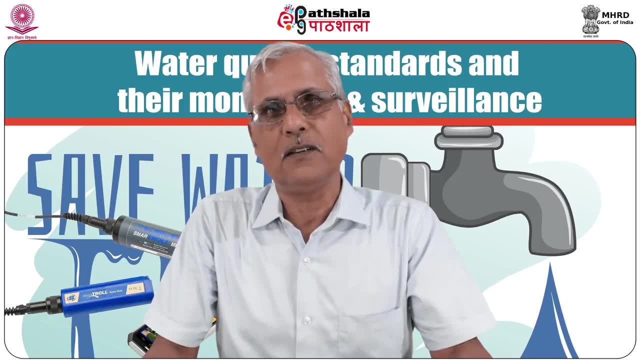 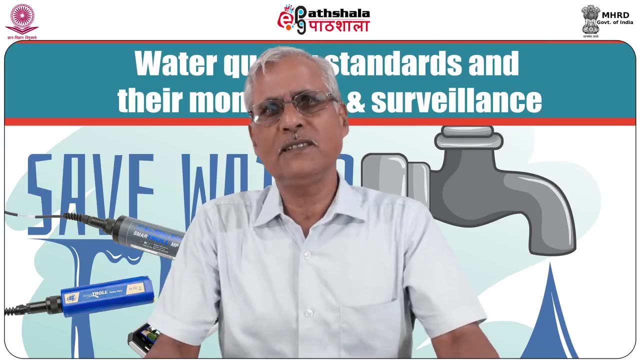 may be used. When a NOAEL or lowest limit value is used instead of a NOAEL, an additional uncertainty factor is normally applied. So this is the system why we are giving considerations of these values Source of uncertainty. uncertainty in derivation of guidelines. values are source of uncertainty. 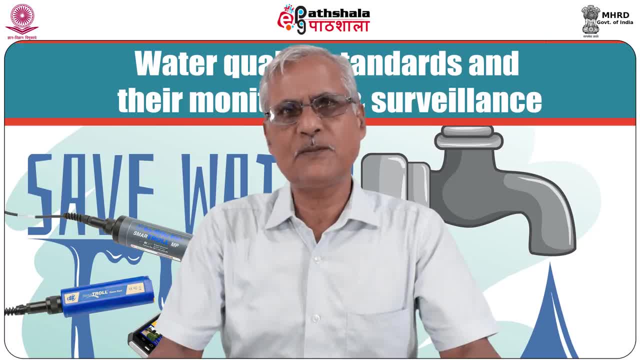 inter-species variation extrapolating from experimental animals to human, uncertainty factor is 1 to 10, inter-species variation accounting for individual variations within humans: 1 to 10. and adequacy for studies of databases: 1 to 10,. nature and severity of 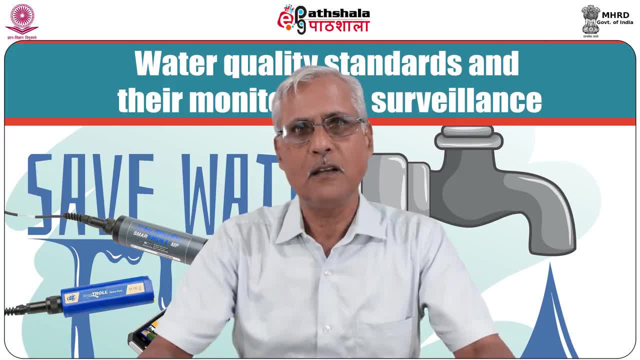 effect 1 to 10.. So these two are taken benchmark dose if appropriate data are available for dose response relations. in modeling, BMDLs are used as an alternative to NOAELs in calculating the health-based guideline values. 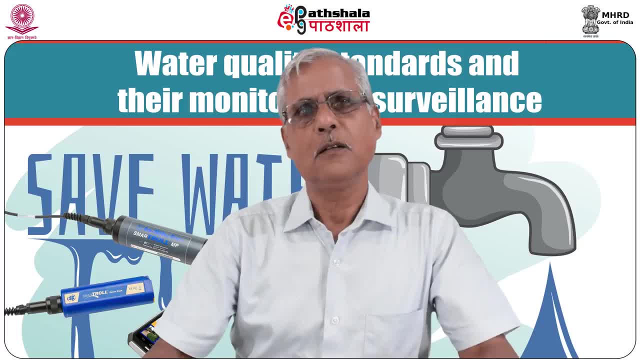 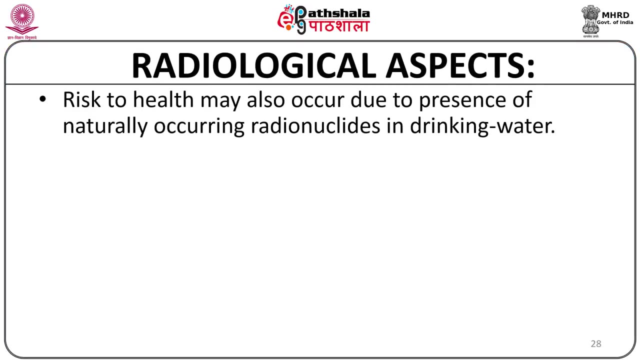 The benchmark, or BMLDL, is the lower confidence limit of the dose that produces a small increase in the level of adverse effects. So radiological aspects- risk of health to health may also occur due to presence of naturally occurring radionucleotides in drinking water. 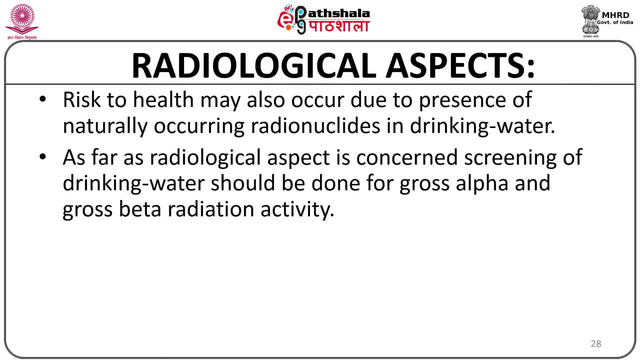 As far as radiological aspect is concerned, screening of drinking water should be done for GRAS-alpha And GRAS-beta radiation activity. levels of screening values do not indicate any immediate risk to health, but it gives clue for further investigation of water. 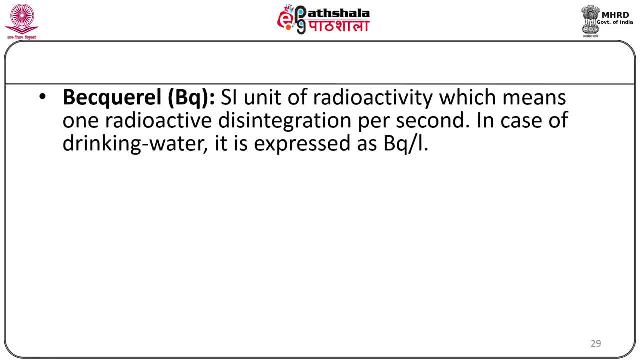 Becquerel BQ. SI unit of radioactivity, which means one radioactive disintegration per second. in case of drinking water, it is expressed as BQ per liter- Effective dose. when radiation interacts with the body, tissues and organs it is used. 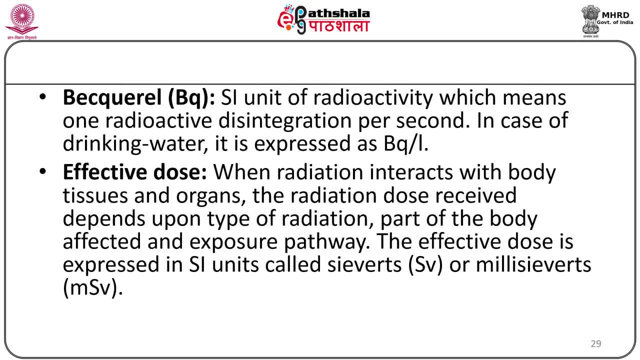 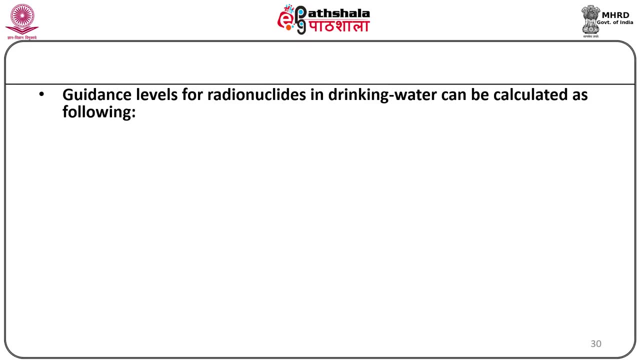 as a test. The radiation dose received depends upon type of radiation, part of the body affected and exposure pathway. The effective dose is expressed in SI units called sieverts or millisieverts. Guiding level of radionucleotides in drinking water can be calculated as following: 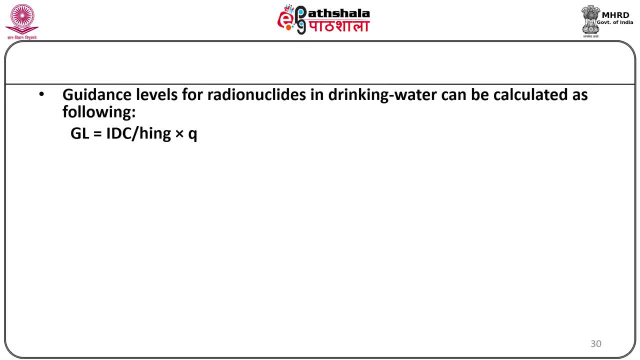 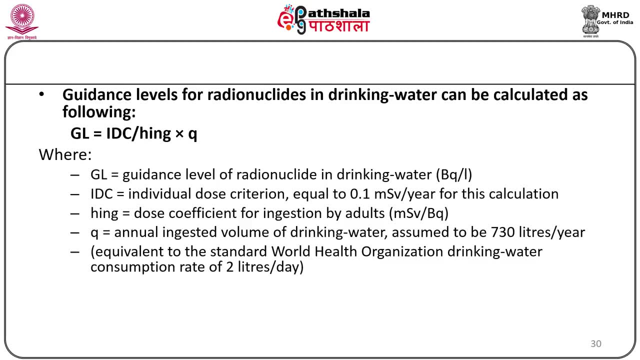 Guiding level is equal to IDC. oblique hinge into Q, where guidance levels of radionucleotides in drinking water is BQ by per liter IDC individual dose criterion equal to 0.1 msb per year. for this calculation Hinge dose coefficient for ingestion by adults, that is msb by BQ and Q, is equal to annual. ingested volume of drinking water assumed to be 732 msb per liter. Guiding level is equal to IDC. oblique hinge into Q, where guidance levels of radioactive radionuclide by hs3K are умmpires to be 730 msb per year, equivalent to the standard. 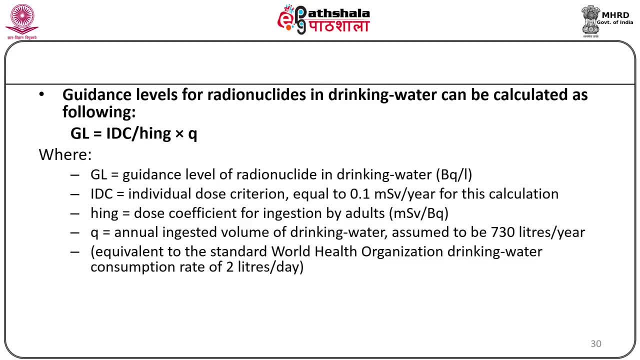 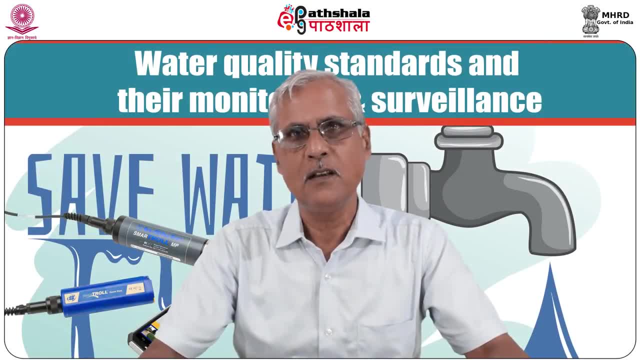 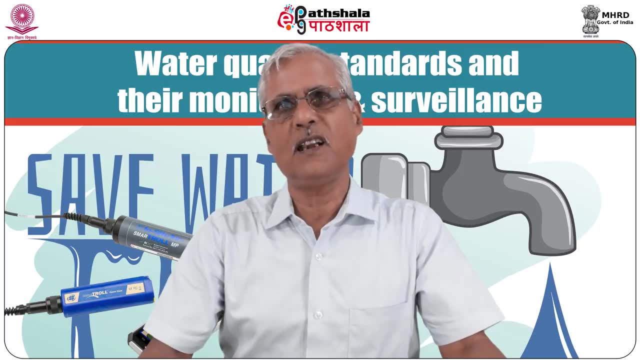 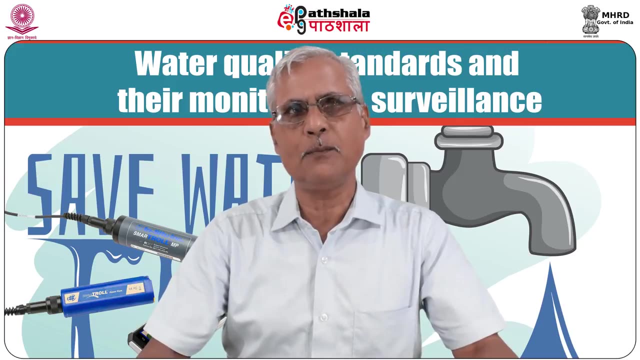 water dilation. drinking water consumption rate of 2 msb per day. Steps for assessment methodology to control radionucleotide: An IDC individual dose criterion of 0.1 msb from one-year consumption of drinking water is adopted In initial screening if the measured activity concentrations are below the screening levels. 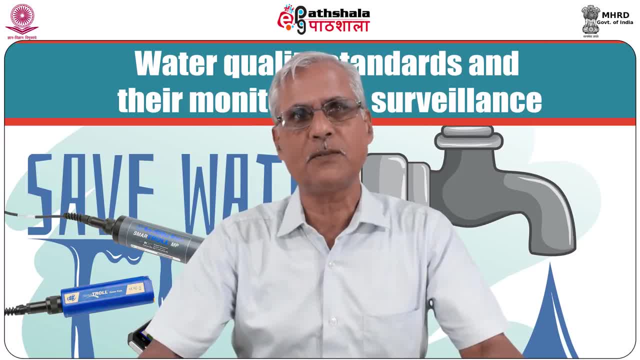 meter for grass alpha activity and 1 bq for grass beta activity. no further action is required If any of the either grass alpha or grass beta activity exceeds the screening level. the concentration of individual radionuclides would be determined and compared with the. 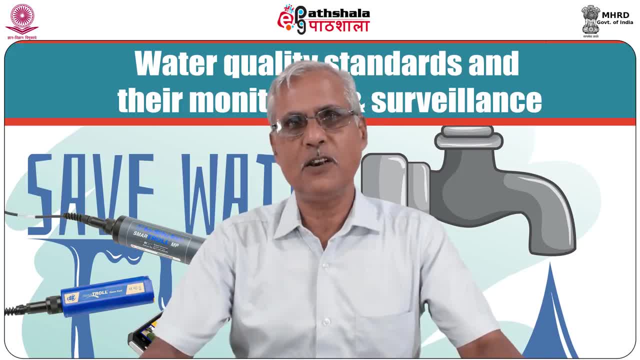 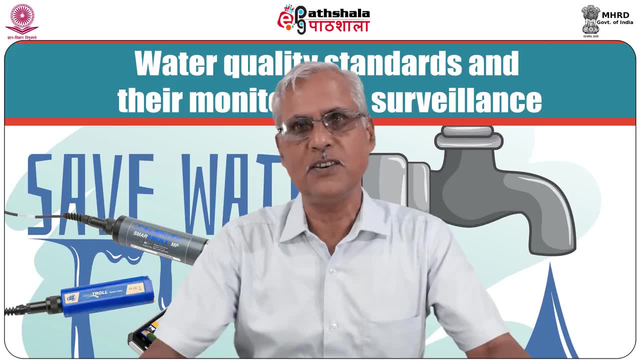 guide dense levels. This further evaluation may indicate either no action is required or further evaluation is necessary before a decision can be made on the need for measurement to reduce the dose. Acceptability, accepts, test order and appearance depends mainly by three parameters: physical, 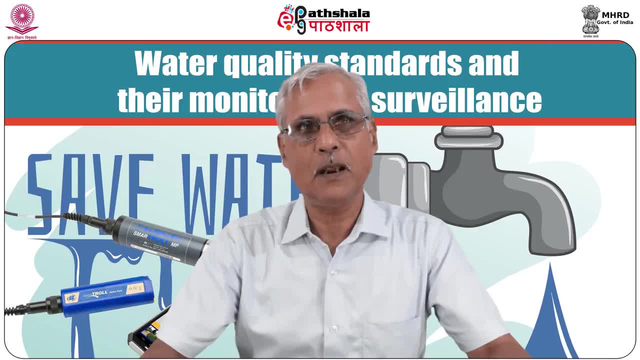 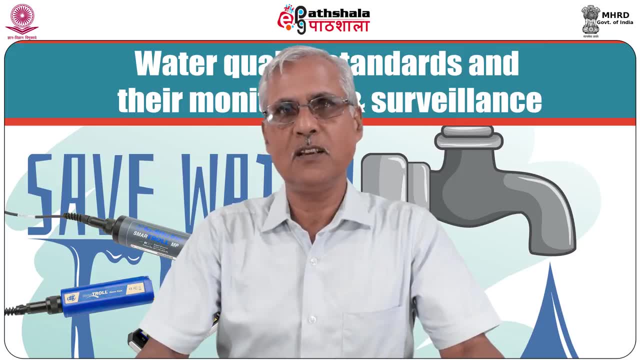 chemical and biological Physical parameters, test order and test and order. water should be free from any objectionable test and orders. Various natural, inorganic, organic, chemical, biological contaminants, sensory chemicals may give rise to test and order. Test and order may also develop during storage and distribution as a result of microbial activity. 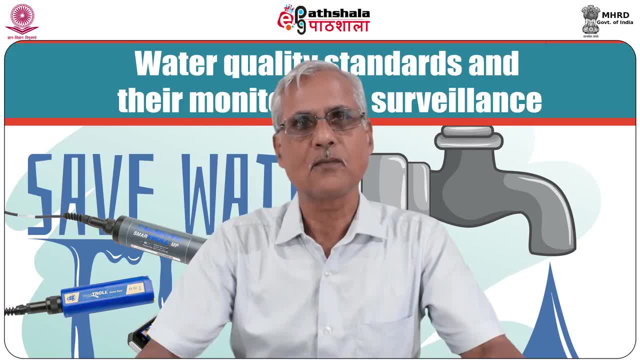 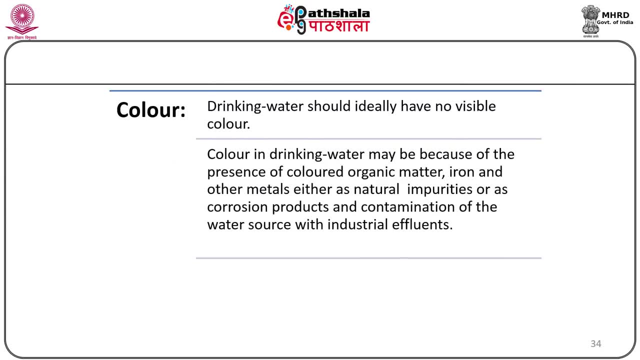 No guideline value has been proposed for test and order. Color drinking water should ideally have no visible color. Color in drinking water may be because of presence of colored organic matter, iron and other metals, either as natural impurities or as corrosion Procedure. 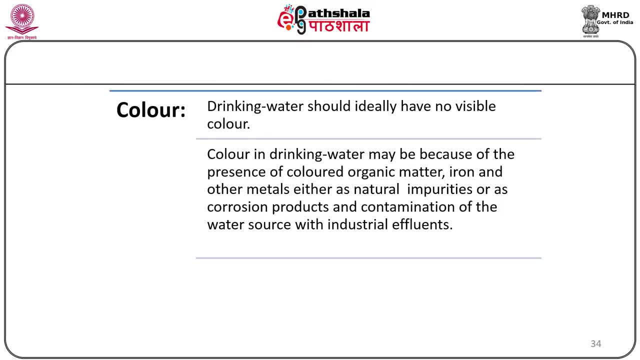 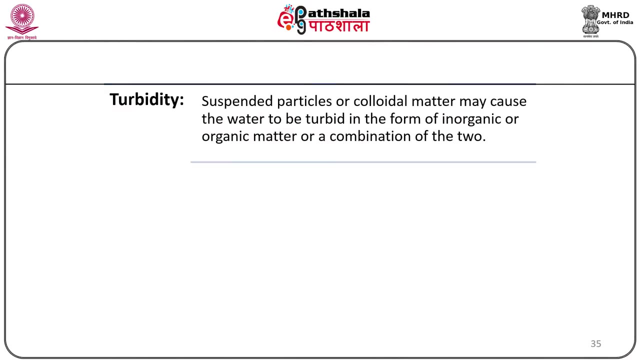 Contamination of water sources with industrial effluents. Color above 15 true color units can be detected in a glass or water. Level of color below 15 TCU are often acceptable to consumers. Turbidity Suspended particles or colloid matter may cause the water to be turbid in the form of inorganic 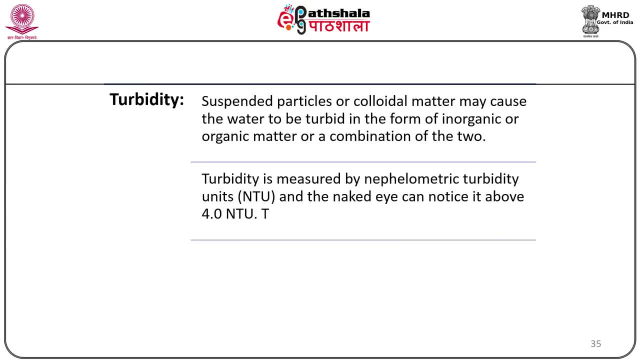 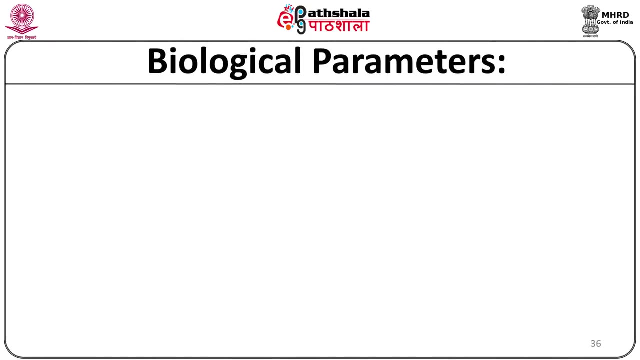 matter, or a combination of the two. Turbidity is measured by naphthalometric turbidity unit and the naked eye can notice it above 4 NTU per T. Turbidity should not be more than 1 NTU, and preferably much lower. 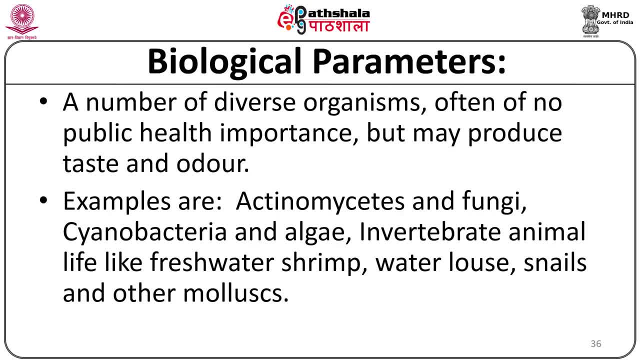 Biological parameters. A number of diverse organisms, Often of different types of organisms, Inorganic matter or a combination of the two. No public health importance but may produce test and order. Examples are actinomycetes and fungi, cyanobacteria and algae. invertebrate animals like fresh. 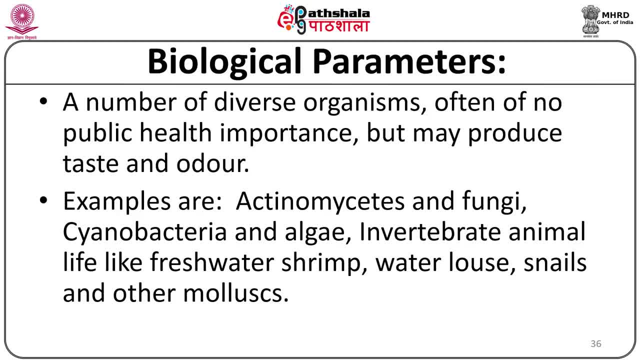 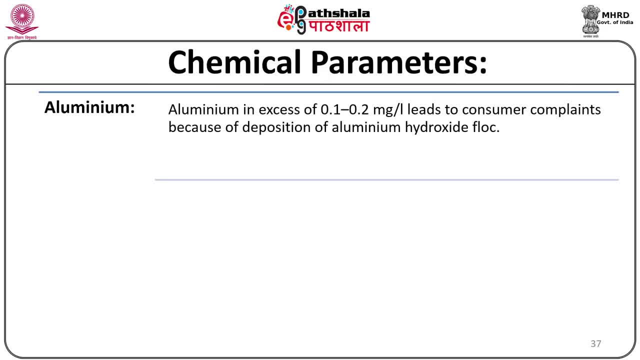 water, shrimp, water louse, snails and other mollusks. Chemical parameters: Aluminium in excess of 0.1 to 0.2 milligram per liter leads to consumer complaints because of deposition of aluminum hydroxide flocculants. 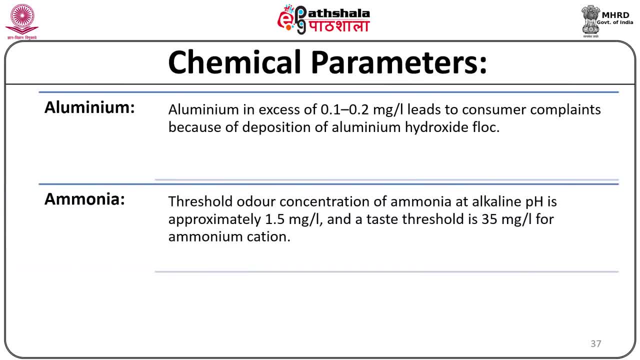 Ammonia Threshold order. concentration of ammonia at alkaline pH is approximately 1.5 milligram per liter and a test threshold is 35 milligram per liter for ammonium cation Chloramines: No order or test is detected for monochloramine at concentration between 0.5 to 1.0 milligram. 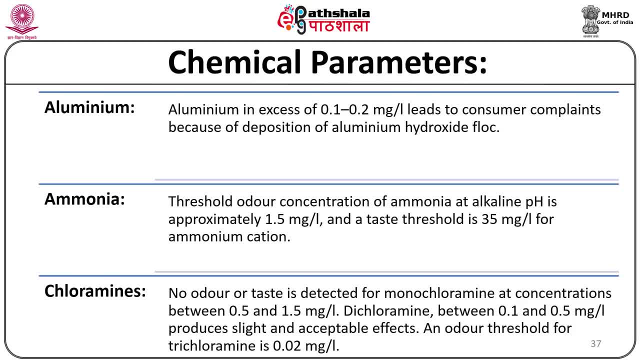 per liter Dichloramine between 0.1 to 0.5 milligram per liter Chloramine: Chloramine at concentration between 0.1 to 0.5 milligram produces slight and acceptable effects. Another threshold for trichloramine is 0.02 per liter. 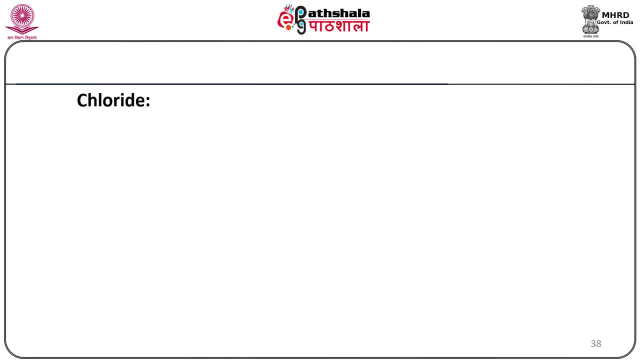 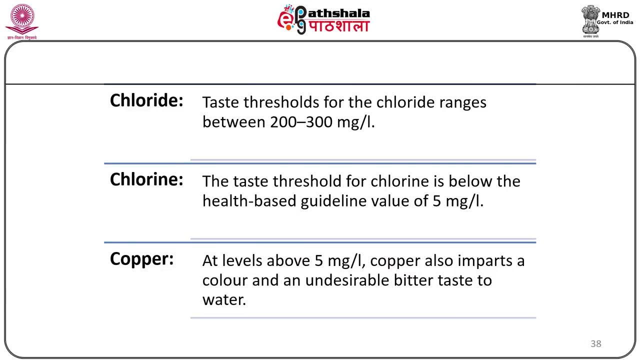 Chloride. Test threshold for chloride ranges between 200 to 300 milligram per liter Chlorine. The test threshold for chlorine is below the health based guideline value of 5 milligram per liter Copper. At levels above 5 milligram per liter copper also imparts a color and an undesirable bitter. 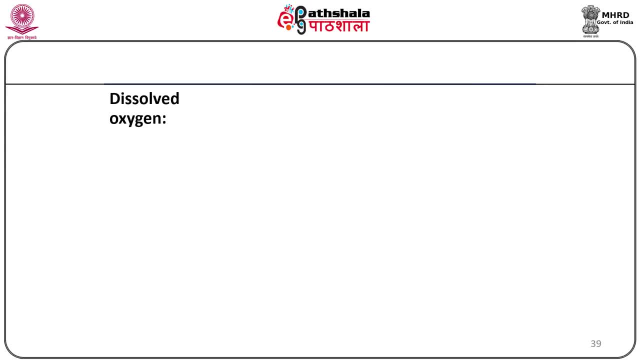 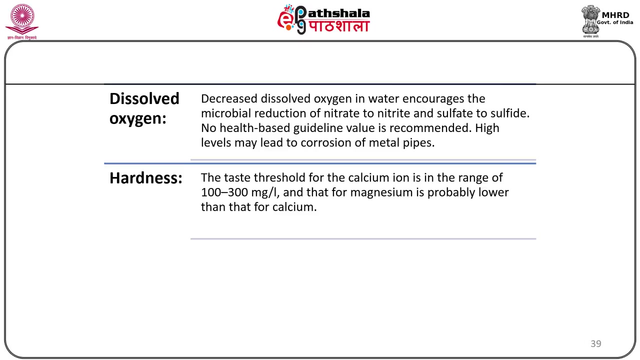 taste to the water. Dissolved oxygen Decreased. dissolved oxygen in water encourages the microbial reduction of nitrate to nitrite and sulfate to sulfite. No health based guideline value recommended. High levels may lead to corrosion Hardness. The test threshold for the calcium ion is in the range of 100 to 300 milligram per liter. 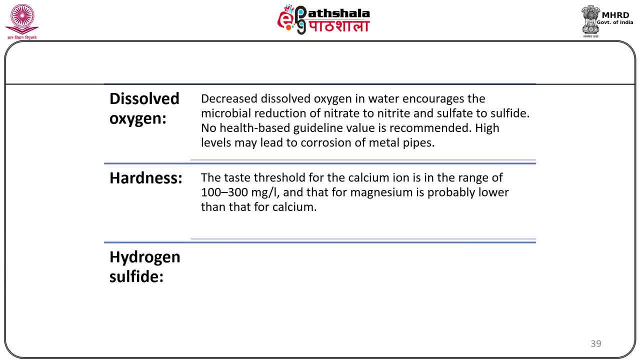 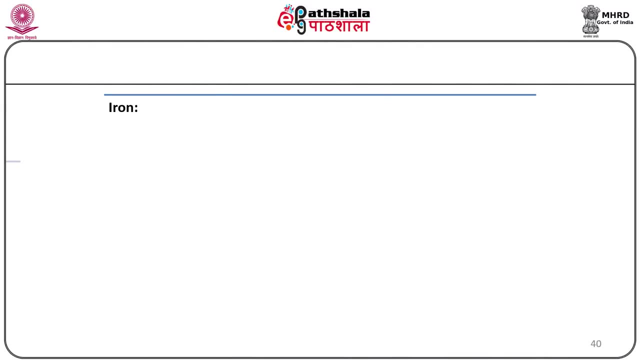 and that for magnesium is probably lower than that of calcium. Hydrogen sulfide: The test and order threshold for a hydrogen sulfide in water are estimated to be between 0.05 to 0.1 milligram per liter Iron Iron does not produce any noticeable change in the test at a concentration below 0.3 milligram. 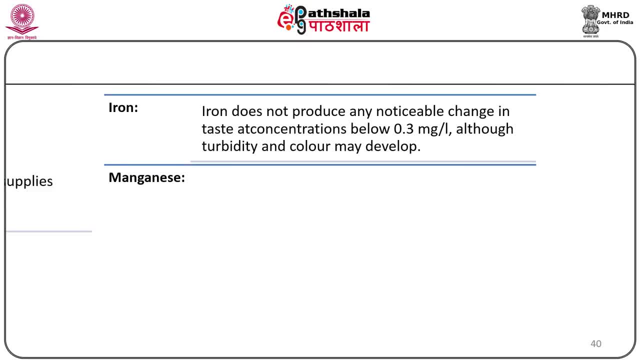 per liter. although turbidity and color may develop Magnesium Above 0.1 milligram per liter, magnesium in water supply causes an undesirable taste. Sodium Test threshold for sodium is about 200 milligram per liter pH. The optimum pH usually ranges from 6.5 to 8.5.. 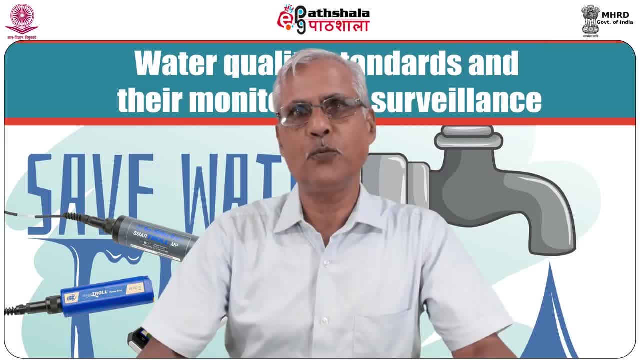 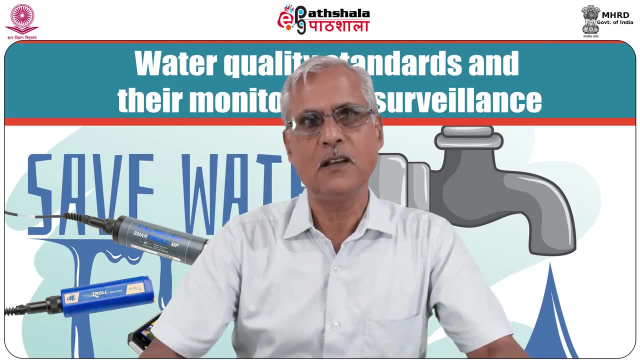 Sulfate. The test threshold ranges from 250 milligram per liter for sodium sulfate to 1000 milligram per liter for calcium sulfate. Total dissolved solids: The palatability of water with total dissolved solids below 60 milligram is considered to. 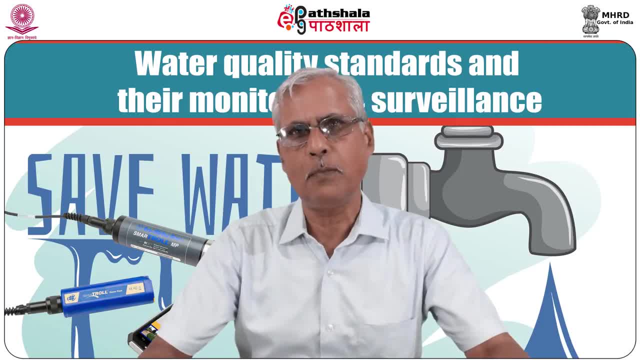 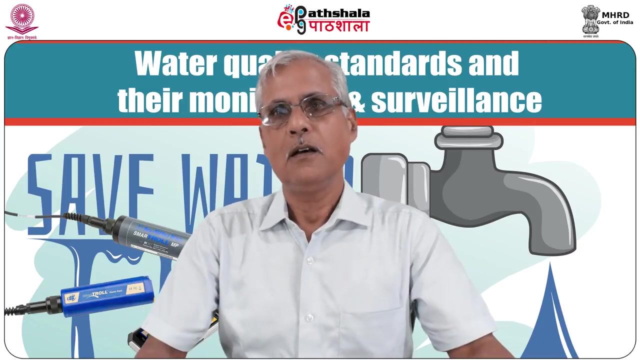 be good, but above 1000 milligram per liter water becomes unpalatable. Zinc- Undesirable taste in water is produced above the threshold concentration of about 4 milligram per liter Zinc sulfate. So once we have discussed the different aspects of quality of water, now we will be switching. 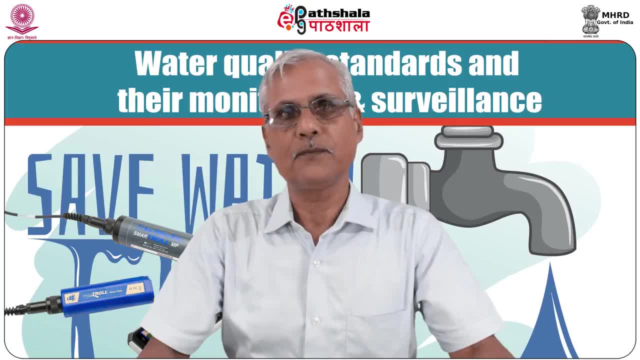 over to surveillance of drinking water quality. Surveillance in relation to quality of drinking water. quality means keeping a good quality of drinking water. Quality means keeping a careful watch at all times, from public health point of view, over the safety and acceptability of drinking water supply. 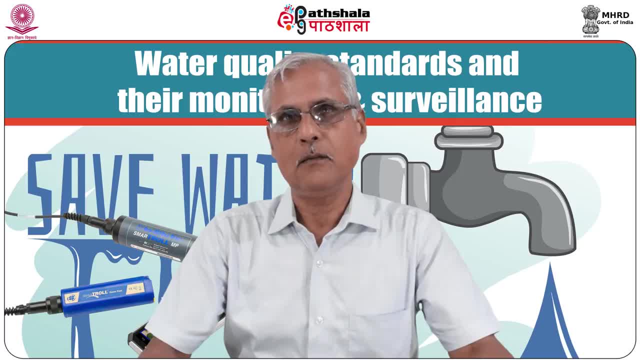 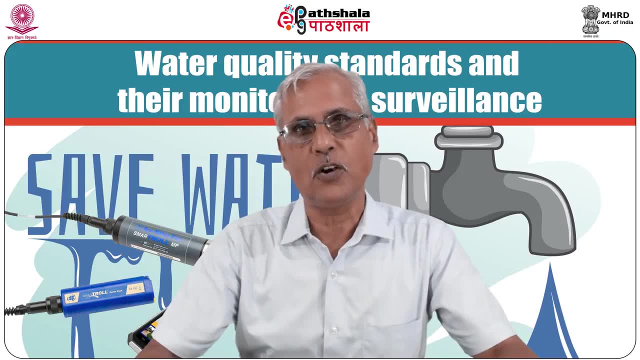 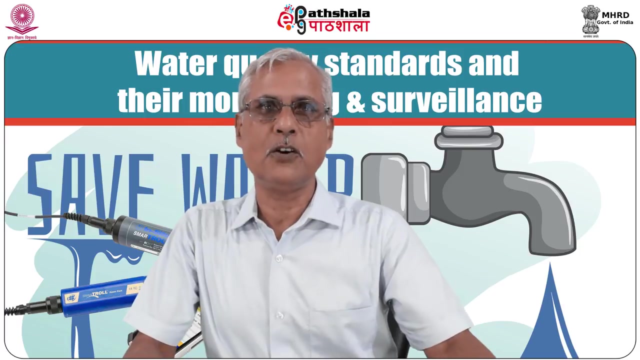 So there are two major issues that comes under the purview of surveillance. One is safety and second is acceptability of drinking water. Key elements are monitoring, sanitary survey, data processing, monitoring of water quality, data processing and evaluation. So in surveillance procedure we are monitoring, we are taking. then we have personality surveys. 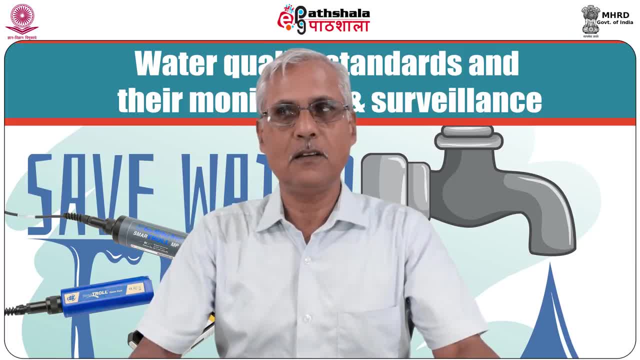 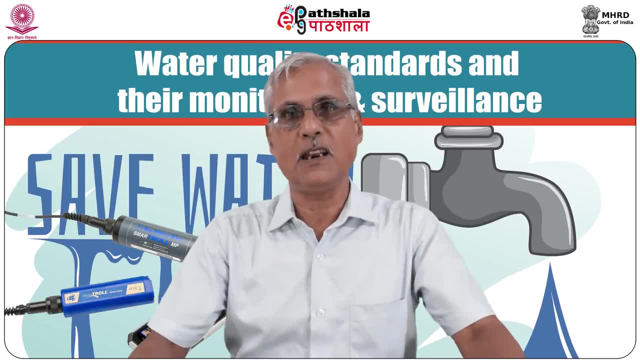 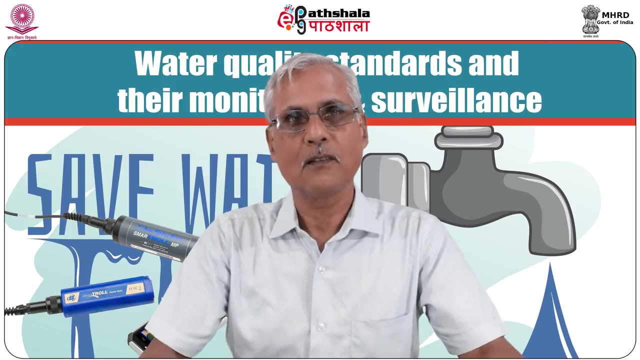 data processing and evaluation. But the ultimate effect of or ultimate purpose of any surveillance activity is to, on top of monitoring there should be an action component, So that so monitoring plus action makes it a surveillance activity. Remedial and preventive action. the last point, remedial and preventive action, is very 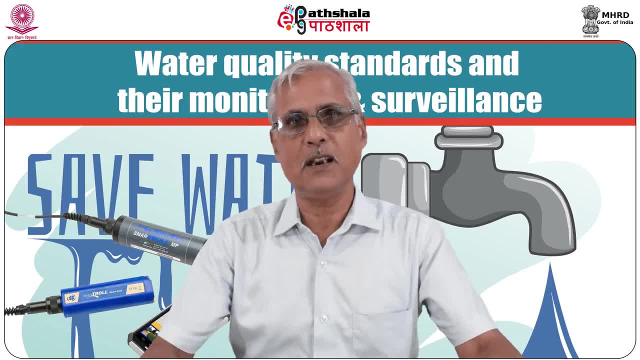 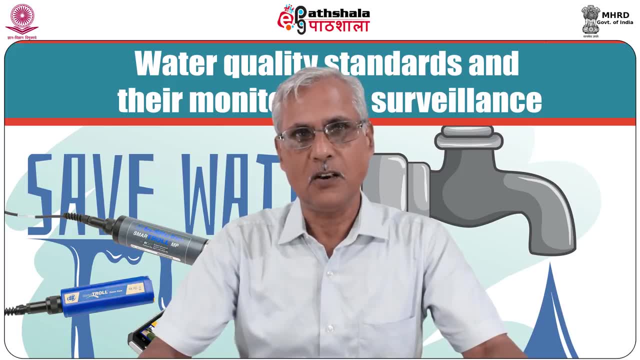 important because if you do not do remedial and preventive action, it is a monitoring activity and it is not a surveillance activity. An institutional analysis is needed: Monitoring- monitoring involves laboratory and field testing of water samples collected from various points in water supply system, including the source, water purification point. 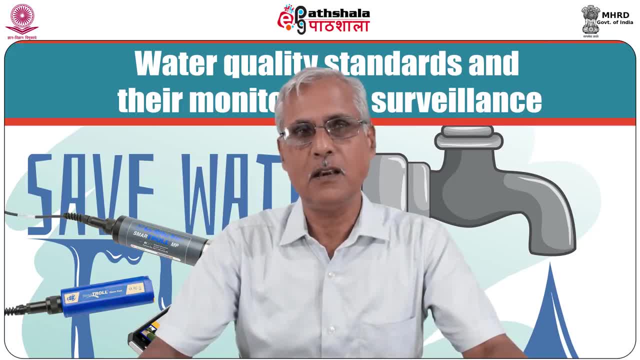 distribution systems, houses and consumer ends. The Central Pollution Control Board is an apex body in the field of water quality management. in India. The water quality monitoring was started in the year 1976 by Central Pollution Control Board with 18 stations on the Yamuna River. 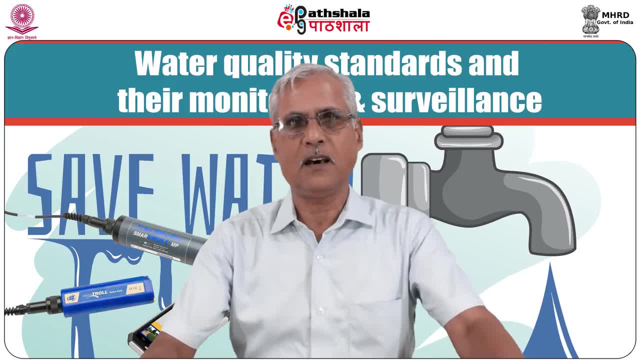 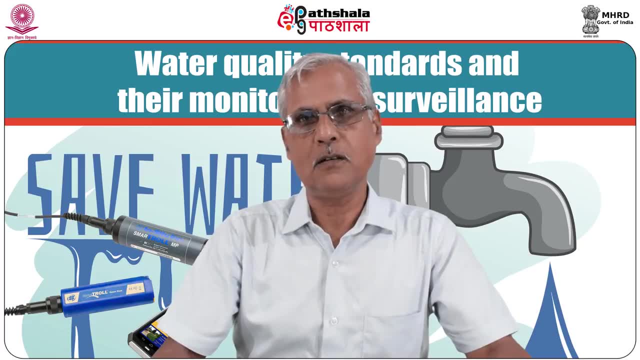 The program has gradually been extended. At present there are 1032 monitoring stations in the country spread over the country. So this is the number of monitoring stations in the country spread over all over all important water bodies. Water sample is taken. the aim of collecting samples is to for assessment of the quality. 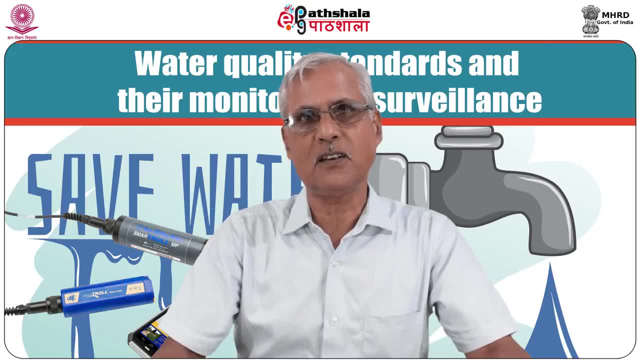 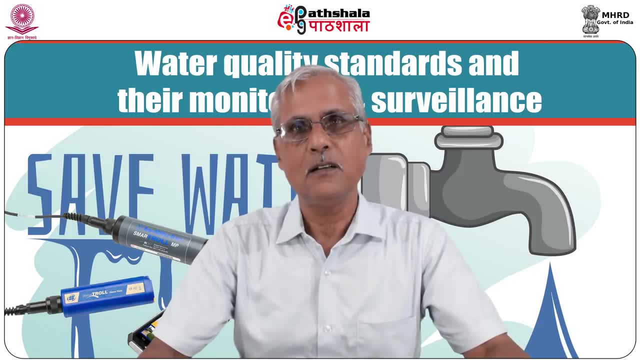 of water from various sources and examination of physical, chemical and bacteriological quality of water. At many places we are doing the most probable number based on mechanism chart, but there are other contaminants, like chemical contaminants, that have a important impact. Segregation of sampling point: samples collected are representative of all the sources from. 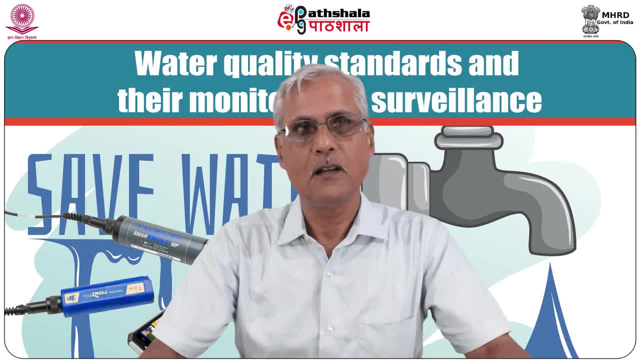 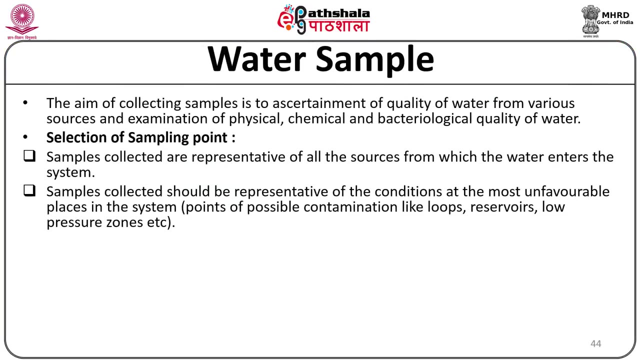 which the water enters the system. Samples collected should be representative of the conditions at the most unfavorable places in the system, points of possible contamination like loops, reservoirs, low pressure zones and so on. Sampling points should be representative of all sources from which the water enters the 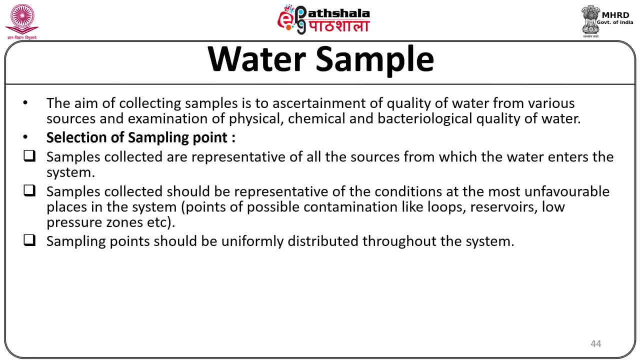 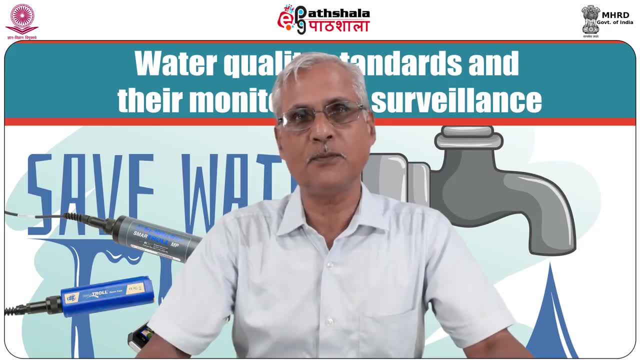 system. Sampling points should be uniformly distributed throughout the system. Many times we do sampling from when water passes through a CTG gradually, then the contamination increases. Samples should also be collected from reservoirs and reserve tanks. At least one sampling point should be there at the clean water outlet from each treatment plant. 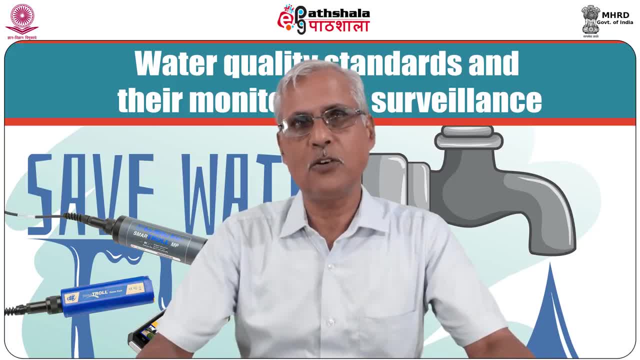 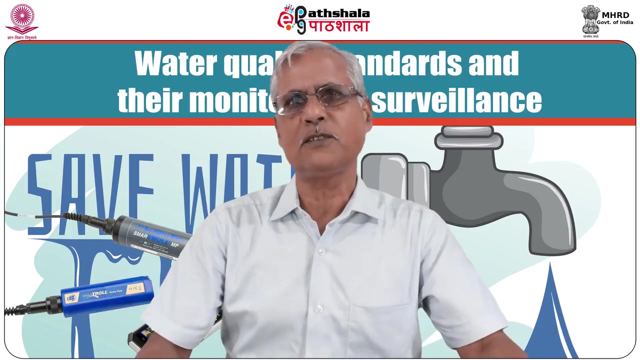 Collection of water sample sampling for bacteriological examination. For bacteriological examination, water samples should be collected in clean, sterilized, narrow-mouthed neutral glass bottles with capacity of 250, 500 or 1000 ml. Colorless or pearl green colored bottles should be preferred, except in case of collecting samples for residual chlorine, where the dark colored bottles must be preferred. 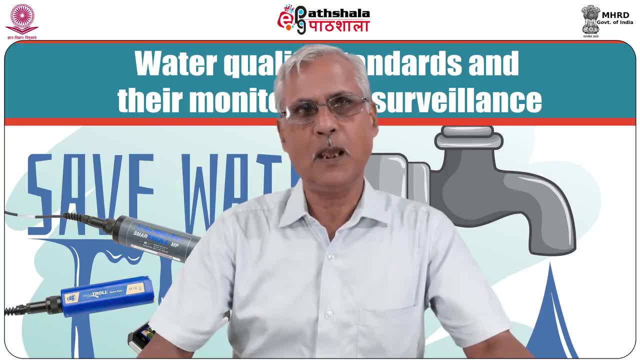 The bottles should be collected in a clean, sterilized, narrow-mouthed neutral glass bottle. This should have a ground glass stopper with an overlapping rim and the stopper should be relaxed by an intervening strip of paper between stopper and neck of the bottle. 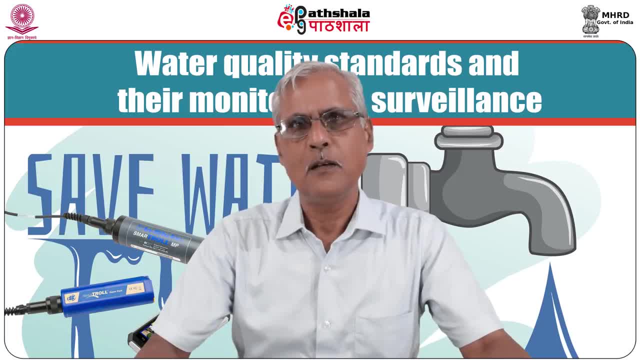 The stopper and neck of the bottle must be protected by paper parchment cover or thorny aluminum paper. Sterilization of the bottle should be done in an autoclave at 1 Kg per cm2 pressure for 15 minutes. The water from which sample is collected. 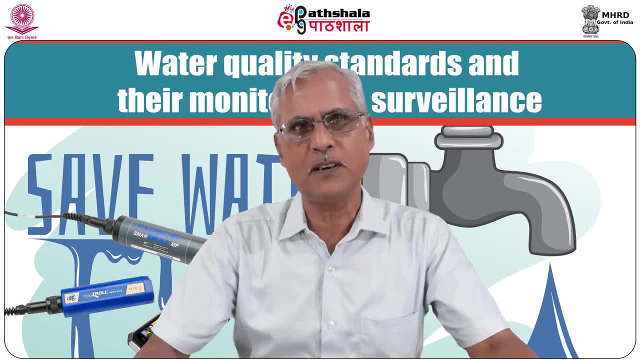 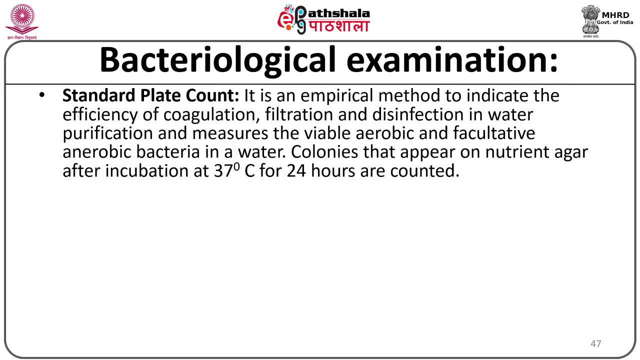 contains residual chlorine alkylamine at 0.2 ml of 10%. sodium thiosulfate, sodium sulfate- to the bottle to neutralize this substance and therefore the bottle is sterilized. Bacteriological examination is an important component. standard plate count: It is an. 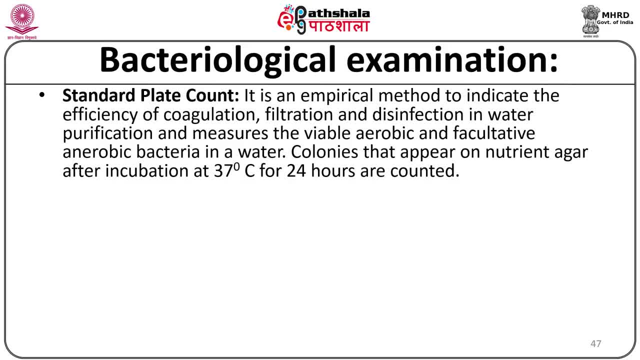 empirical method to indicate the efficiency of coagulation, filtration and disinfection in water purification and measures the viable aerobic and facultative anaerobic bacteria in water colonies that appear on nutrient tagger after incubation at 37.4% or counted. 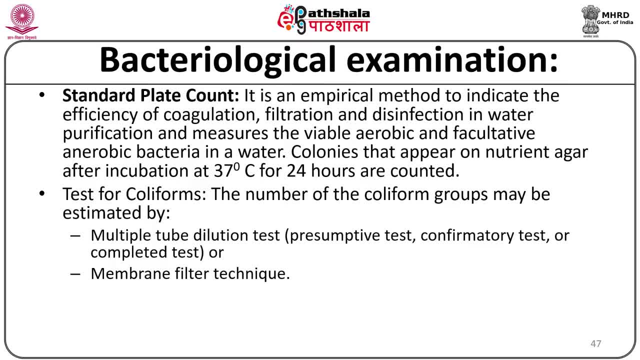 Test for coliforms. the number of coliform group may be estimated by multiple treatment, dilution method, the empty test, confirmatory test and completed test or membrane filtration technique and charts are available which can be taken. 坊 most probable number: Multiple tube dilution test: MTD In analysis of water: at least 3. 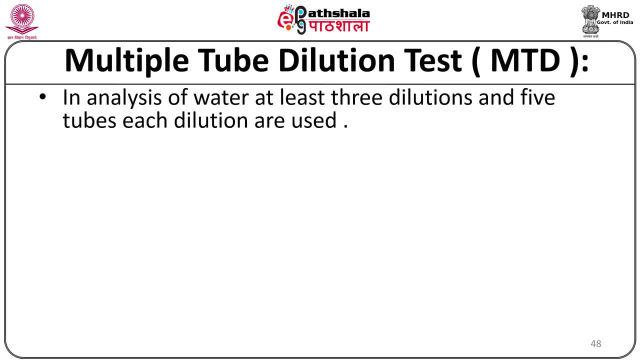 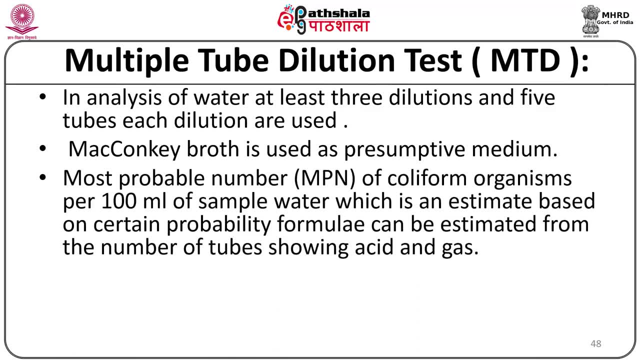 milli dilutions of 5 tubes each dilution are used. Most probable number, coliform, means per 100 ml. the sample water which is estimated based on certain probability- formerly can be estimated from the number of tubes showing acid and gas value for a given sample can be obtained using MPN tables and this has been given one table. 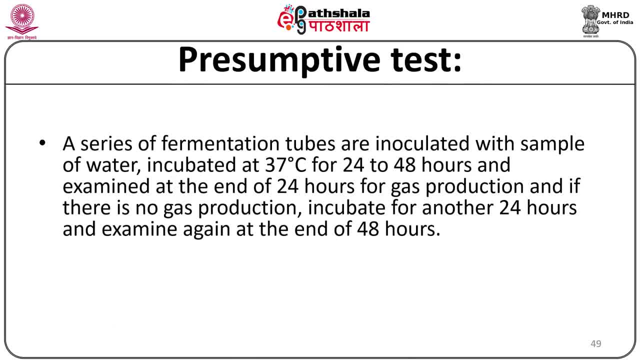 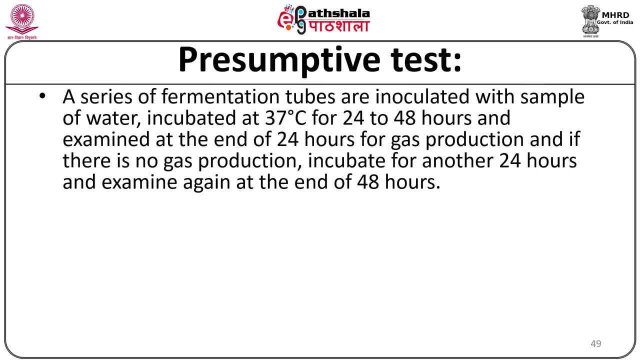 is given by magnetic chart Resume to test. a series of fermentation tubes are inoculated with samples of water, incubated at 37 degree centigrade for 24 to 48 hours and examined at the end of 24 hours for gas production. and there is no gas production, incubate for another 24 hours and examine. 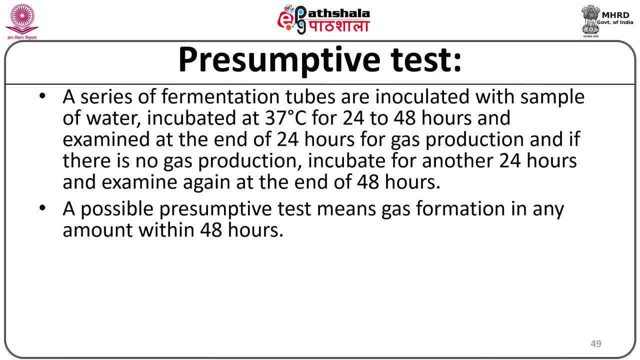 again at the end of 48 hours. A possible presumptive test means gas formation, any amount within 48 hours. If no gas formation occurs at the end of 48 hours, the test is considered negative Conformity test. the test is performed using all primary fermentation tubes showing gas. 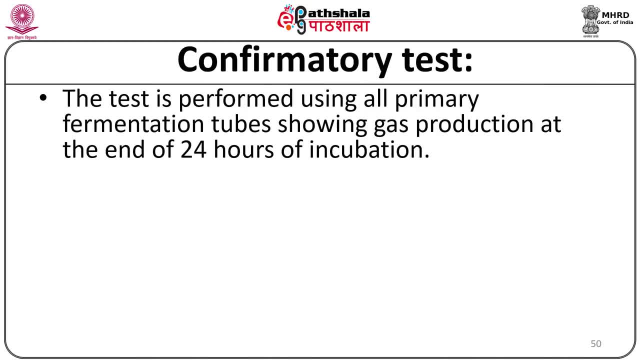 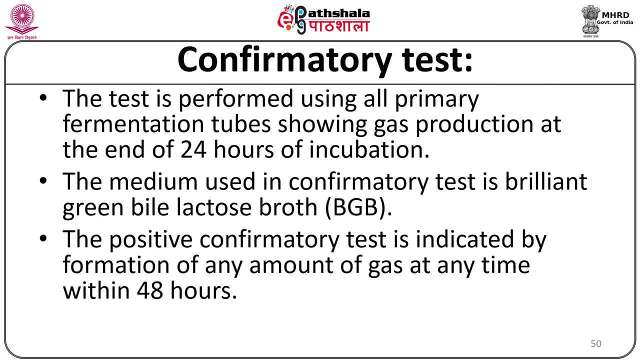 production at the end of 24 hours of incubation. The medium used in conformity test is a medium Conformity test is brilliant green bile lactose growth. The positive conformity test is indicated by formation of any amount of gas at any point within 48 hours. 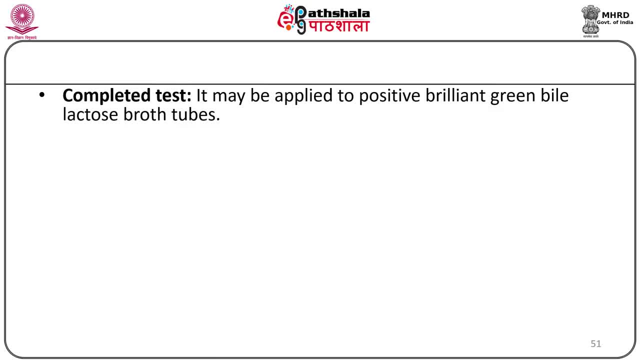 Completed test. it may be applied to positive brilliant green bile lactose growth tubes By measuring membrane filtration technique. by using membrane filtration technique, results can be obtained within 24 to 48 hours. M-indobroth is used as a medium in membrane filtration techniques. 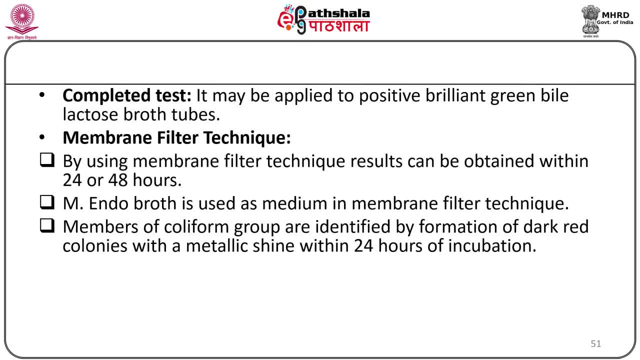 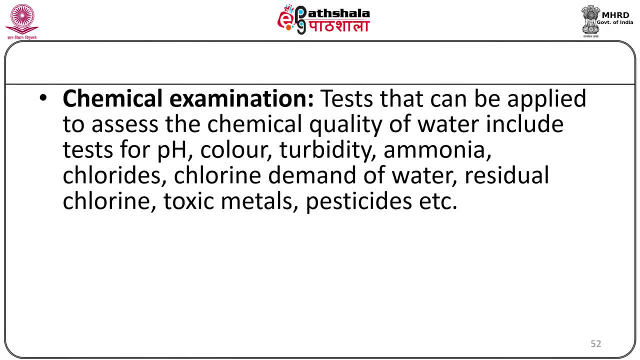 Members of coliform group are identified by formation of dark red colonies with a metric sign with 24 hours of incubation. Chemical examination: the test that can be applied to assess the chemical quality of drinking water include, for test for pH, color turbidity, ammonia, chloride, chlorine demand. 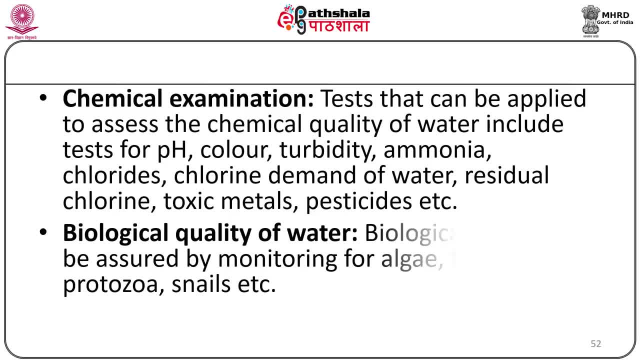 of water, residual chlorine, toxic metals and pesticides. The test can be performed at the end of 48 hours. Bacteriological quality: of what the biological unit can quality can be assessed by monitoring for algae, fungi, yeast, protogravins, snails and so on. 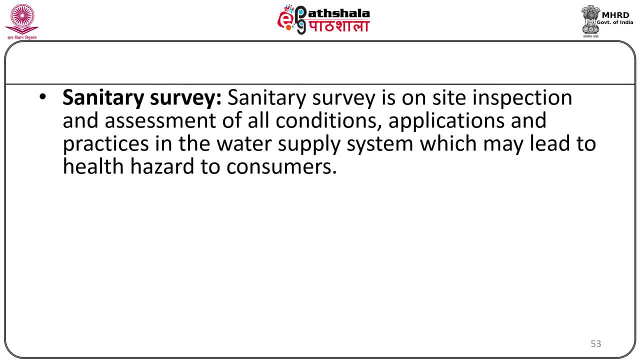 Sedentary survey. sedentary survey is on the site inspection, assessment of all conditions, applications and practices in water supply system which may lead to health hazards to consumers. This also gives us action points, Data processing and evolution the huge data generated by monitoring in sedentary survey. 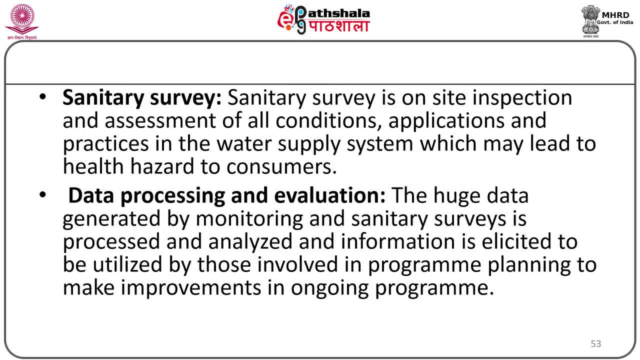 which may lead to health hazards to consumers. This also gives us action points: Data processing and evolution: the huge data generated by monitoring in sedentary survey which may lead to health hazards to consumers. This also gives us action points: Data processing and evolution: the huge data generated by monitoring in sedentary survey. 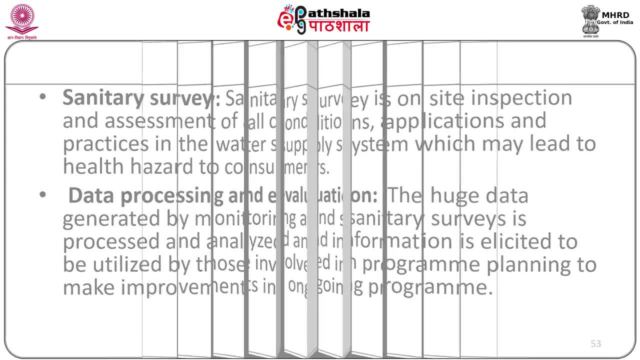 which may lead to health hazards to consumers. This also gives us action points: Data processing and evolution: the huge data generated by monitoring in sedentary survey which may lead to health hazards to consumers. This also gives us action points: Data processing and evolution: the huge data generated by monitoring in sedentary survey. 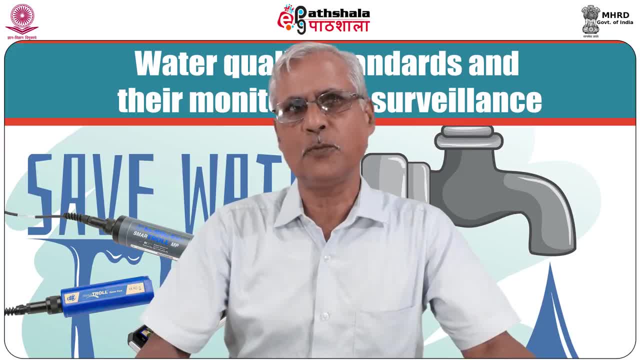 which may lead to health hazards to consumers. This also gives us action points: Data processing and evolution: the huge data generated by monitoring in sedentary survey which may lead to health hazards to consumers. This also gives us action points: Data processing and evolution: the huge data generated by monitoring in sedentary survey. 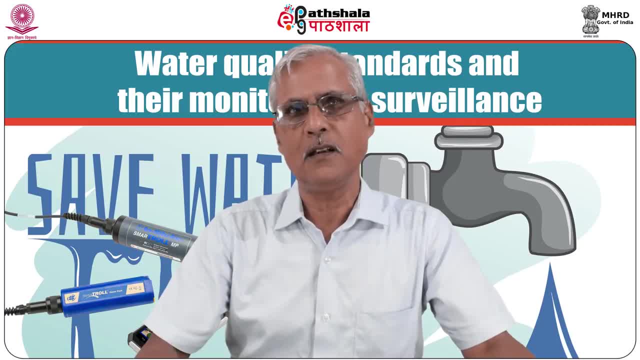 which may lead to health hazards to consumers. This also gives us action points: Data processing and evolution: the huge data generated by monitoring in sedentary survey which may lead to health hazards to consumers. This also gives us action points: Data processing and evolution: the huge data generated by monitoring in sedentary survey. 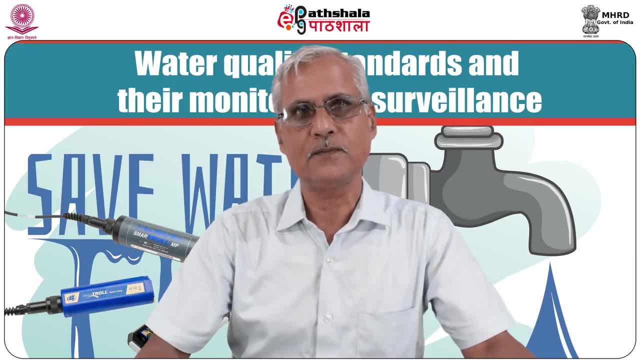 which may lead to health hazards to consumers. This also gives us action points: Data processing and evolution: the huge data generated by monitoring in sedentary survey which may lead to health hazards to consumers. This also gives us action points: Data processing and evolution: the huge data generated by monitoring in sedentary survey. 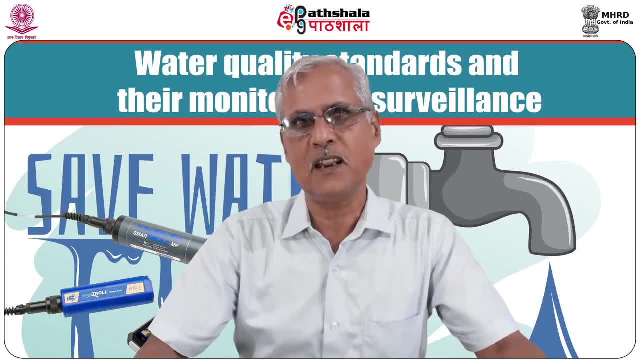 which may lead to health hazards to consumers. This also gives us action points: Data processing and evolution: the huge data generated by monitoring in sedentary survey which may lead to health hazards to consumers. This also gives us action points: Data processing and evolution: the huge data generated by monitoring in sedentary survey. 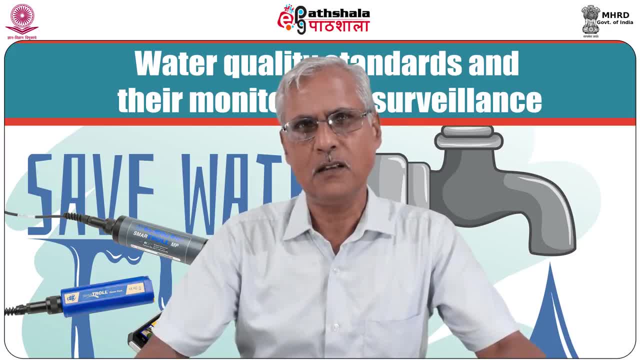 which may lead to health hazards to consumers. This also gives us action points: Data processing and evolution: the huge data generated by monitoring in sedentary survey which may lead to health hazards to consumers. This also gives us action points: Data processing and evolution: the huge data generated by monitoring in sedentary survey. 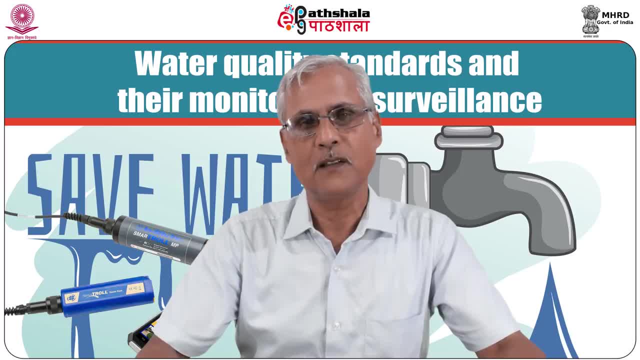 which may lead to health hazards to consumers. This also gives us action points: Data processing and evolution: the huge data generated by monitoring in sedentary survey which may lead to health hazards to consumers. This also gives us action points: Data processing and evolution: the huge data generated by monitoring in sedentary survey. 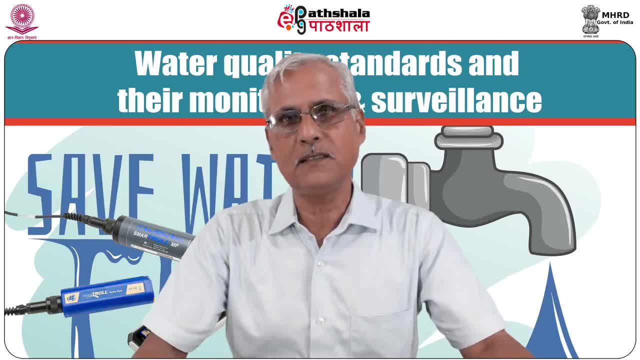 which may lead to health hazards to consumers. This also gives us action points: Data processing and evolution: the huge data generated by monitoring in sedentary survey which may lead to health hazards to consumers. This also gives us action points: Data processing and evolution: the huge data generated by monitoring in sedentary survey. 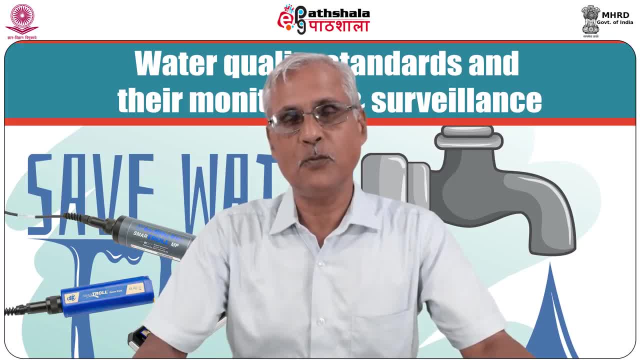 which may lead to health hazards to consumers. This also gives us action points: Data processing and evolution: the huge data generated by monitoring in sedentary survey which may lead to health hazards to consumers. This also gives us action points: Data processing and evolution: the huge data generated by monitoring in sedentary survey.